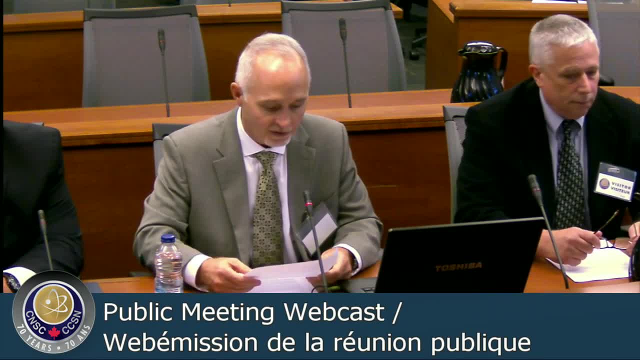 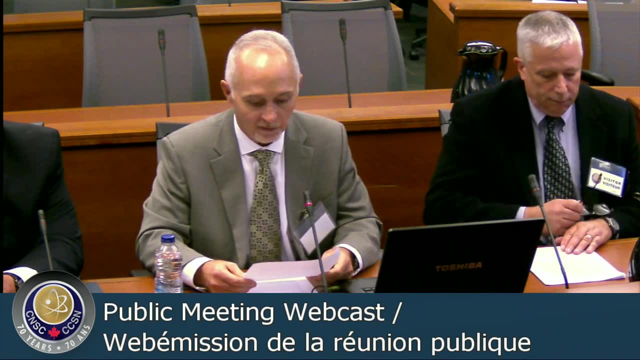 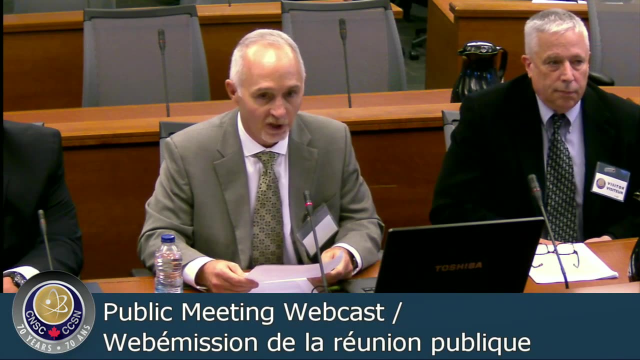 Head of White Shell Laboratories Closure Project. Behind me is Jim Buckley, Director of the Near Surface Disposal Facility. This presentation is a follow-up to a commitment made to the Commission during our April appearance, where we committed to provide a broad overview of the decommissioning and waste management program at CNL. We appreciate the Commission scheduling. 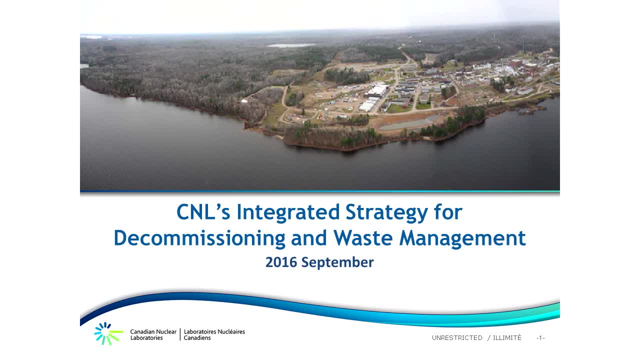 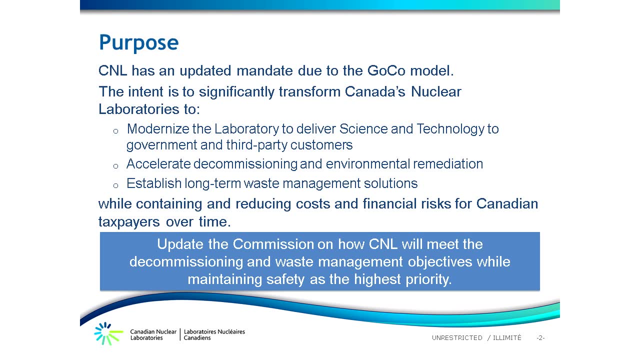 the time for us to be here today. As you may recall, we have a new mandate associated with the transition to a government-owned contractor-operated or GOCO model at CNL. First and foremost, our mission is to modernize. 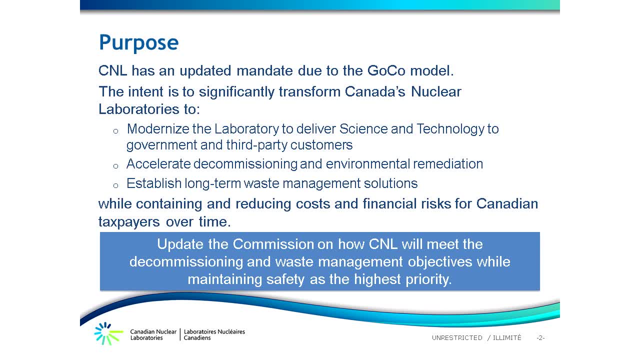 the infrastructure, capabilities and approach to deliver science and technology to the government and to third-party customers. To support this, we need to be able to provide a broad overview of the decommissioning and environmental remediation and establish long-term waste management solutions, while 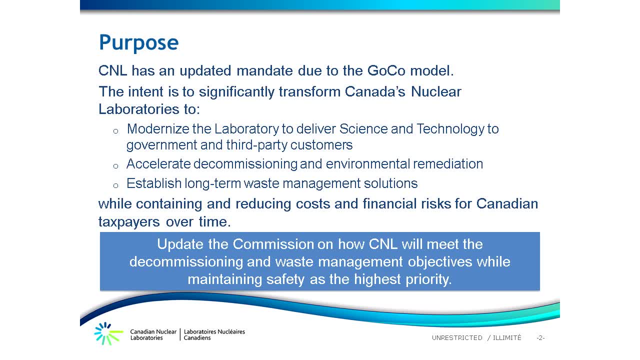 reducing costs and the financial risk to the Canadian taxpayers. This presentation is to update the Commission on how the decommissioning and waste management organization will safely meet these objectives. We are engaged in many activities that will bring us before the Commission over the next few years. 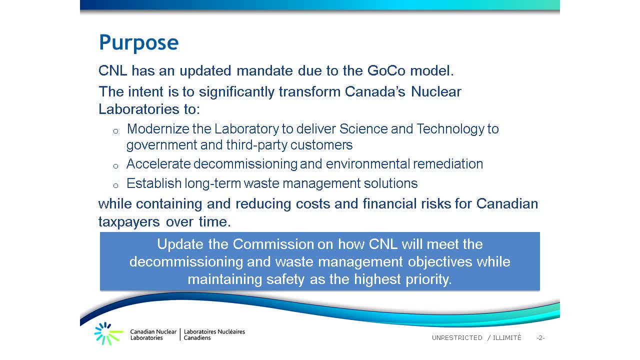 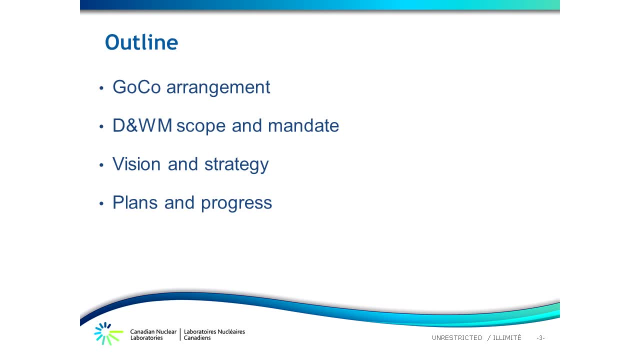 So today's meeting is to provide the big picture prior to any specific licensing hearings. The outline for this section of the presentation is to refresh the Commission on the government-owned contractor-operated model at CNL, describe the scope of decommissioning and waste management. 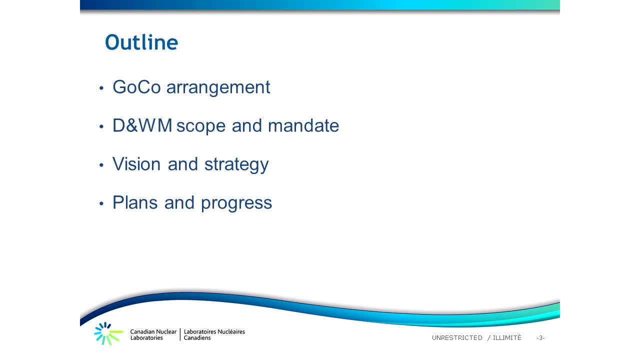 within the context of the new mission, cover the vision and strategy of the new mission and the strategy to safely perform the work and provide plans and progress at Chalk River. After I finish my portion of the presentation, I'll turn over to Pat Daley to review the Nuclear Power Demonstration Project. 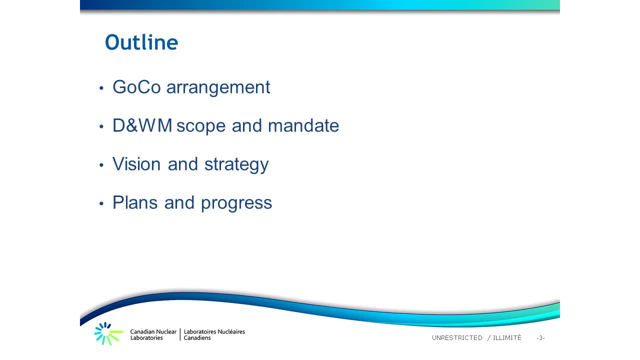 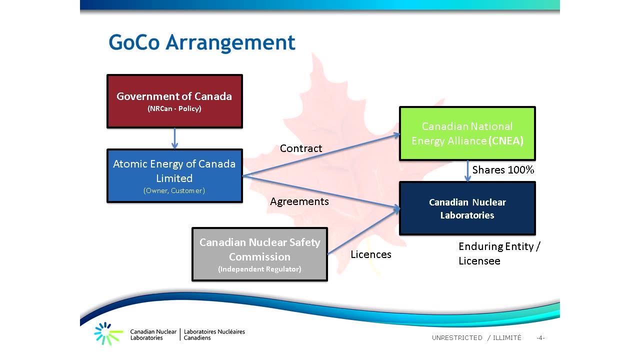 and to Dan Coyne to provide an update on the Whiteshell Labs Closure Project. In the GOKO structure, CNL is the licensee. In the GOKO structure, CNL is the licensee. We operate the facilities and undertake activities under the authority of the licenses issued by the CNSC. 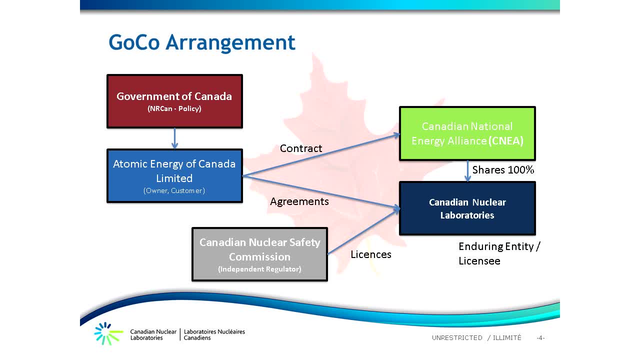 CNL's shareholder is Canadian National Energy Alliance, who holds the contract with AECL. AECL oversees the contract and CNL's performance on behalf of the Government of Canada. AECL also retains ownership of the sites, facilities, assets, intellectual property and the decommissioning liabilities. 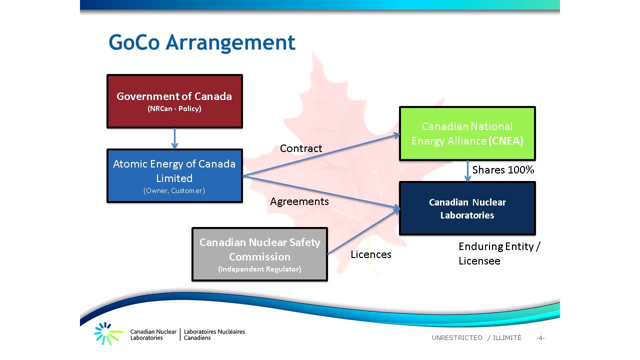 AECL takes policy direction from the federal government through Natural Resources Canada. I'd like to point out the slide states agreements plural between AECL and CNL. While there is a site operating contract for CNL in general, there are also two separate target cost contracts for Whiteshell and for the nuclear power demonstration projects. 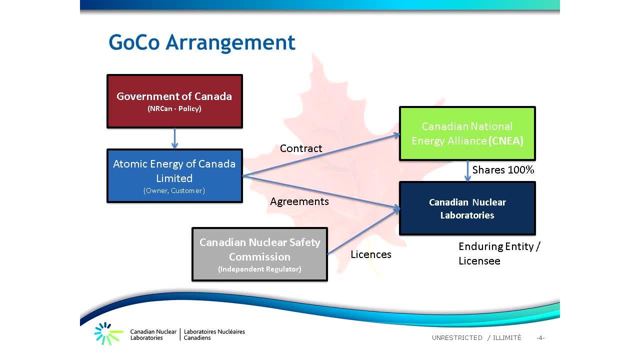 I want to assure the Commission that, as a licensee, we understand our responsibilities for safety and protection of the environment and that these are our highest priorities. I can also assure the Commission that our contracts with AECL are aligned with these priorities. Thank you. 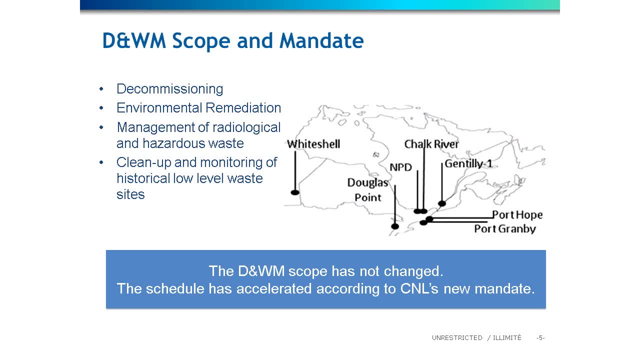 The DWM organization at CNL has a broad scope, both in terms of physical geography and the nature of the work. We are actively commissioning Chalk River site facilities that are no longer needed for operation. We are decommissioning Whiteshell Labs site in Manitoba. 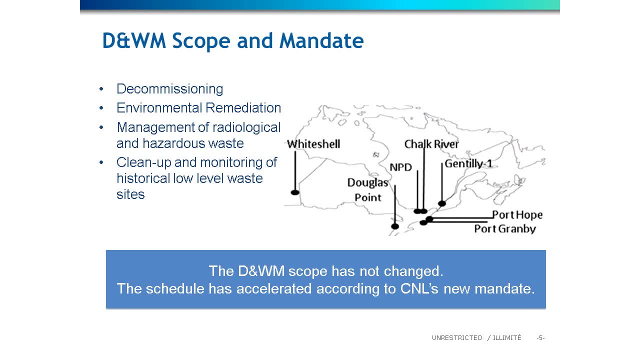 We are responsible for the prototype power reactors at Douglas Point, John T One and the Chalk River site. The nuclear power demonstration reactor is the first of the prototype reactors to undergo complete decommissioning. We are responsible for environmental remediation at the CNL sites. 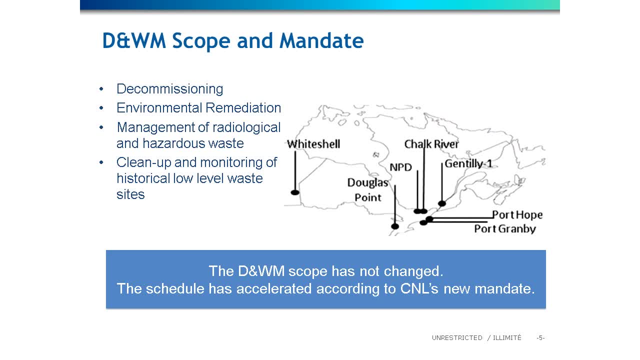 and for managing CNL's radioactive and hazardous wastes, including wastes arising from both past and current operations, as well as from some commercial sources. We are also responsible for the cleanup of historical low-level radiological waste sites at Port Hope and Port Granby. 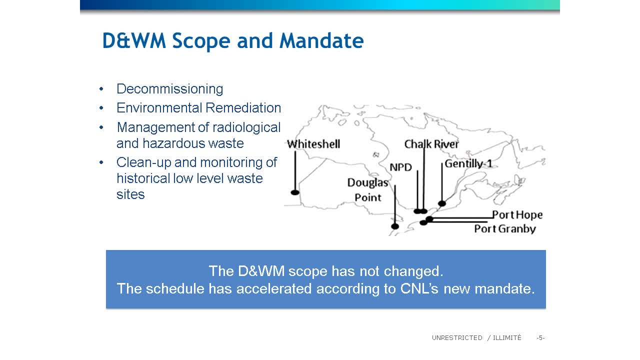 Our low-level radioactive waste management office is responsible for monitoring historical waste facilities in numerous locations along the northern transportation route and the greater Toronto area. As an example, our staff also traveled to Fort McMurray after the devastating fire there to check on the Beacon Hill long-term waste management facility. 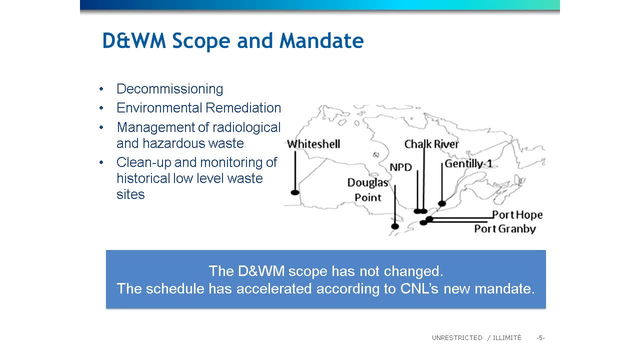 As with CNSC's determination, our organization confirmed there are no safety concerns with this site as a result of the fire. The nuclear liabilities being addressed by the GOCO contract have not changed from previously, but the schedule has been accelerated with the implementation of the new model. 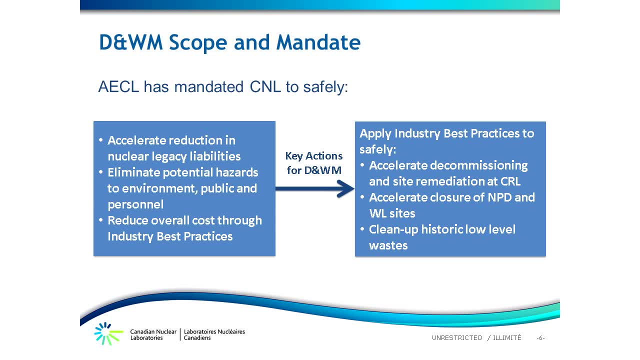 The next slide, please. Decommissioning and waste management's emphasis is on early reduction and elimination of hazards and liabilities, With safety as the highest priority. we will accelerate decommissioning and site remediation at Chalk River, Nuclear Power Demonstration and at Whiteshell sites. 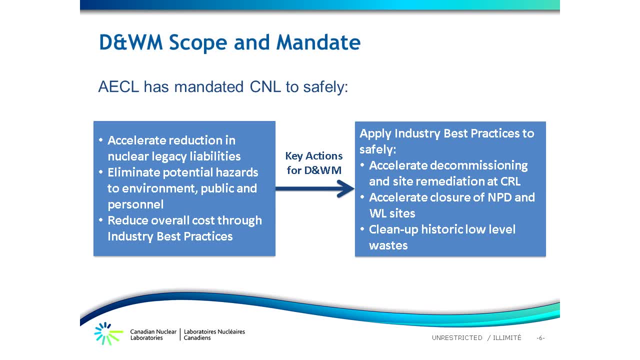 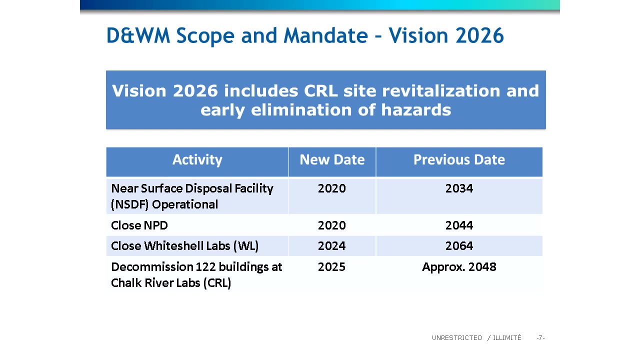 and we will clean up historical low-level waste sites. We fully understand the licensing approvals required to support this work and we are engaged with CNL on this. We will work with CNSC staff to support the multiple concurrent licensing efforts underway. The vision of a revitalized Chalk River laboratory has been coined: Vision 2026,. 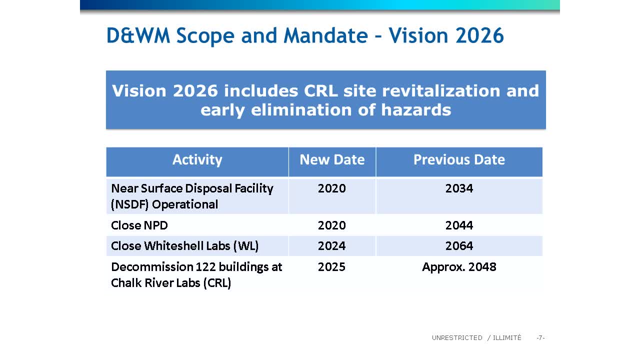 which is now being incorporated into our five- and ten-year plans. These plans include both revitalization and the elimination of legacy liabilities. The key DWM activities and the ones we'll talk about more in detail today are shown on the slide. 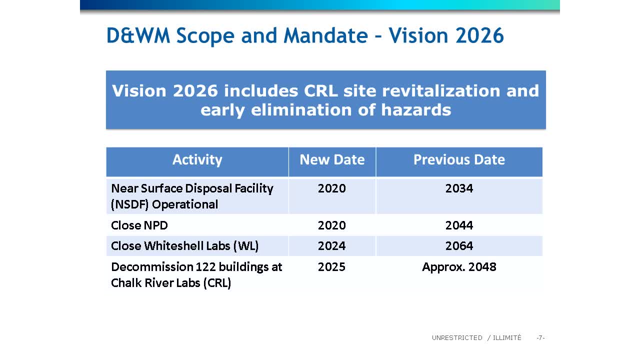 As you can see from the table, we are advancing the schedule across the board, in some cases by decades. This will support revitalization and renewal of the lab and eliminate hazards, instead of having to manage hazards in temporary methods for many years At Chalk River. the previous plan indicated we'd have a one-year plan. 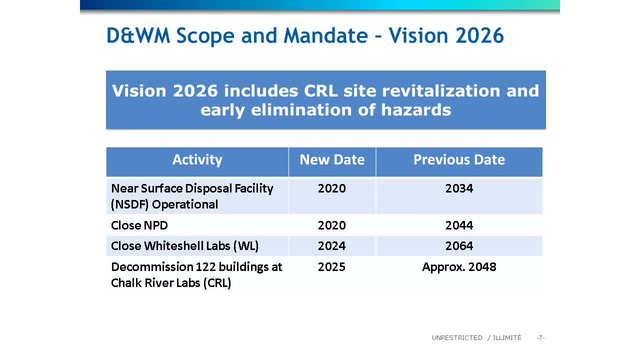 and we have a waste disposal facility in place by 2034.. Our current plan is to have the near-surface disposal facility operational 14 years earlier in 2020.. This is a key enabling facility essential to support our plan for decommissioning activities. 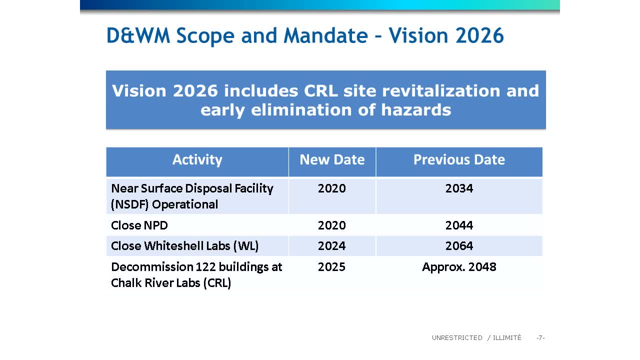 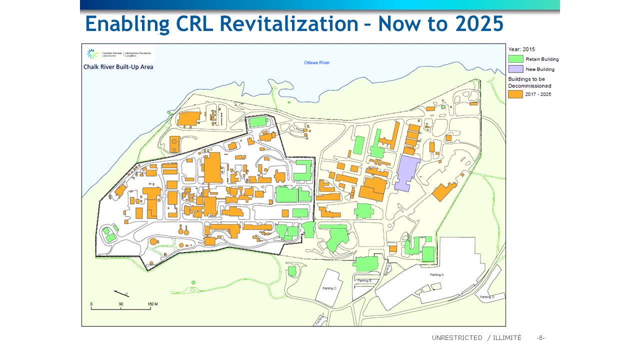 which reduces the hazards and paves the way for site revitalization. The acceleration of the nuclear power demonstration in the Whiteshell sites will have more detail later in this presentation. This slide and the next illustrate how we will revitalize the Chalk River site. 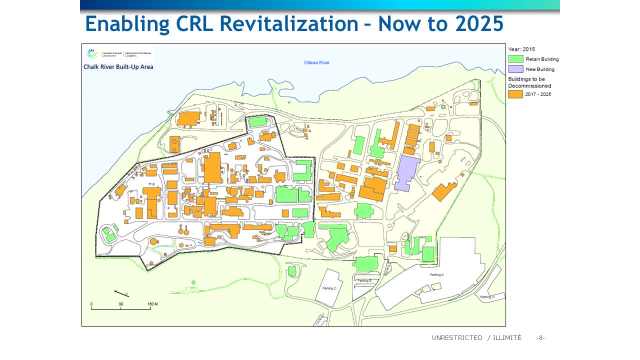 This is a map of the current built-up area of the Chalk River site, showing the buildings in the active area on the left, as surrounded by the dark line which is the protective fence, and the administration area on the right. Over the 10 years of the contract, our plan is to decommission and remove. 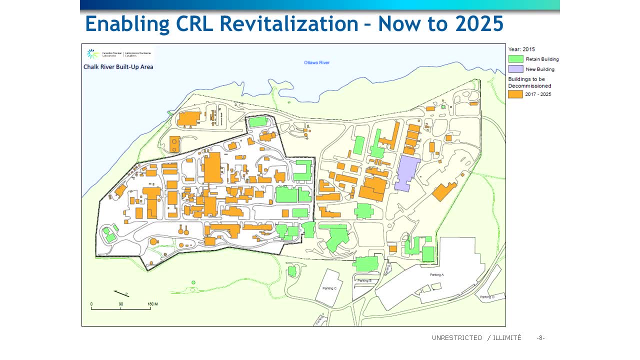 122 structures at the Chalk River site, as illustrated by all the buildings which are in orange. At the same time, we will continue to operate many facilities and we will build new ones to support the overall C&L mission. The one new building shown in purple on this slide. 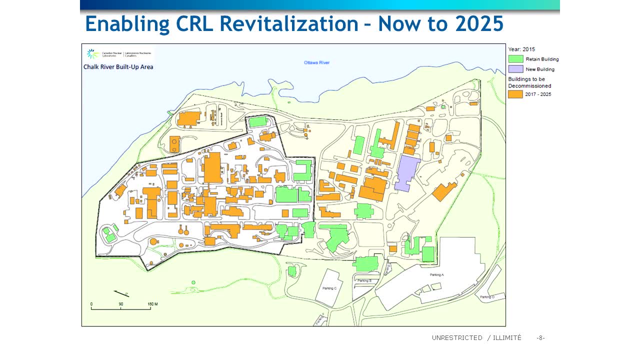 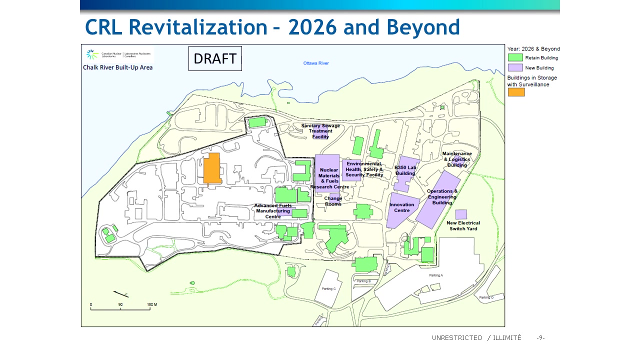 is a new state-of-art laboratory for chemistry and materials research. Construction has just recently been completed. This lab will allow us to take down older buildings where this type of work has been taking place in the past. The next slide shows a vision of what a revitalized Chalk River site. 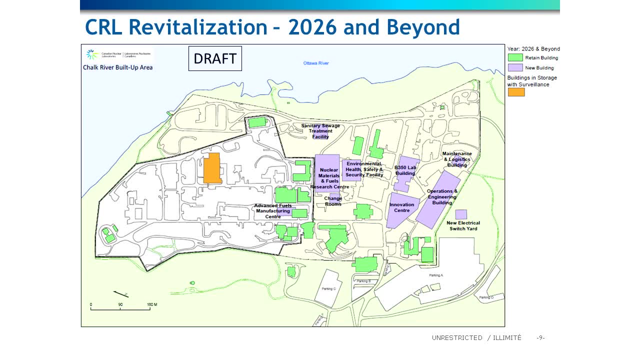 might look like, While our plans are not firm. we envision multiple new laboratories to deliver on science and technology and new, upgraded infrastructure By 2026,. the orange buildings from the previous slide will be gone, with one exception. The one exception is the NRU reactor, which will remain in storage. 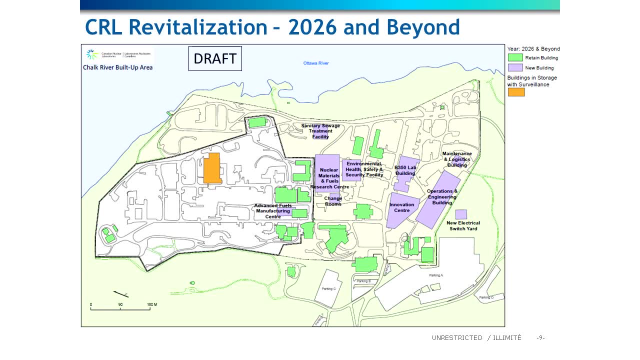 with surveillance until a later date for decommissioning. For completeness, here are some of the other major activities DWM will be performing, including: completion of the Port Hope Area Initiative. completion of the treatment and disposal of the stored liquid waste at Chalk River site. 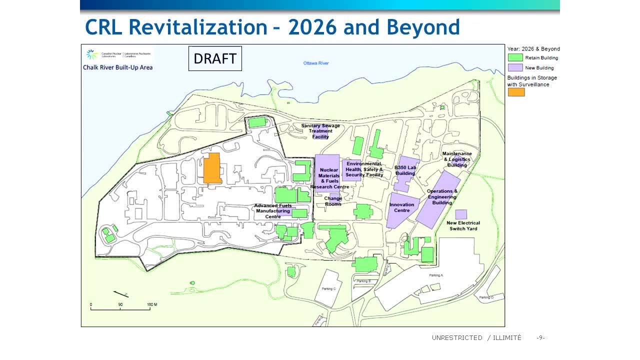 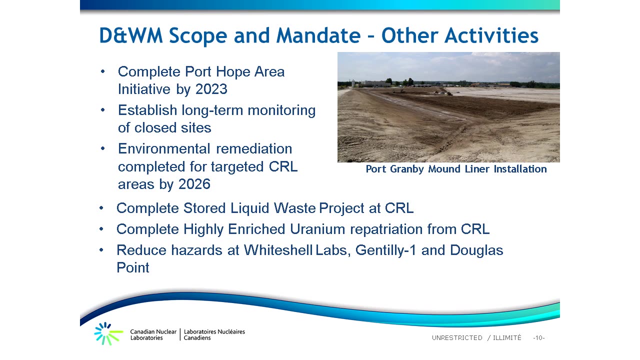 completion of the highly enriched uranium repatriation. Additionally, we will continue risk reduction at John T One and at Douglas Point prototype reactor sites To safely achieve the 2026 vision. decommissioning and waste management has a three-pronged strategy. 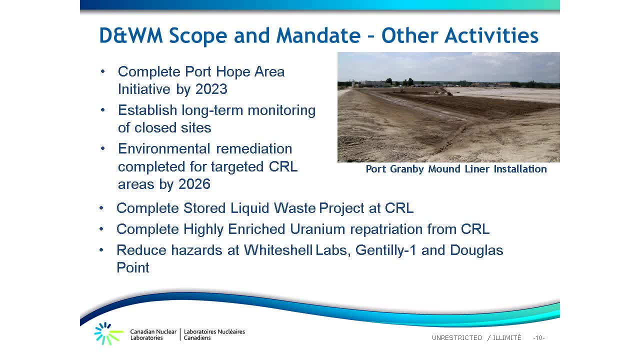 The first element to achieve the strategy is focus, accountability and leadership. The decommissioning and waste management program is in one organization, at Chalk River, reporting to me With two key projects: the white shell, led by Dan Coyne, and nuclear power demonstration, led by Pat Daly. 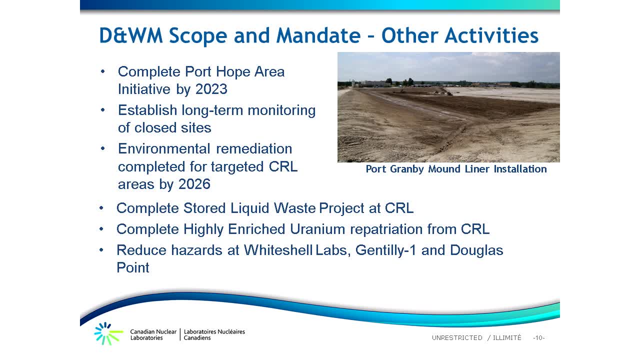 reporting directly to the Chief Executive Officer, Mark Leszczynski, to ensure they get the proper oversight and support they need. We have an excellent group of leaders who have successfully and safely completed similar projects in other locations, And we are working with C&L staff on local knowledge. 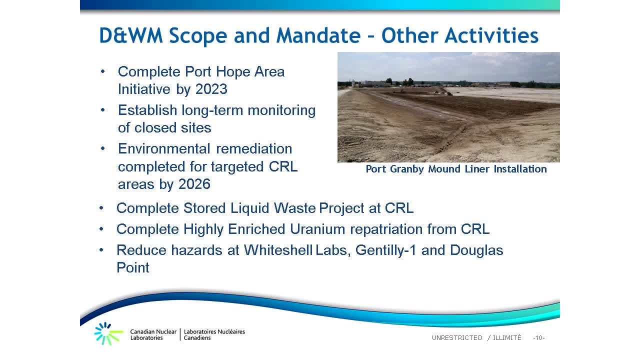 and expertise. We have a clear 10-year plan with contractual incentives and penalties that align with safety first philosophy. We are using an integrated work teams to ensure that the resources are committed to the project's success. The final point I want to emphasize under this part of the strategy: 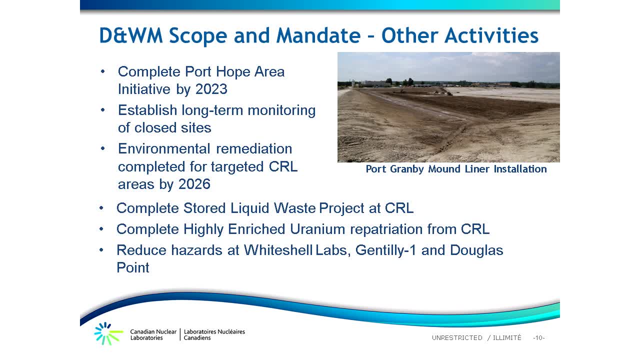 is the people. Implementing DWM strategy requires a significant increase in the resources at the site. We are working to retrain, redeploy C&L staff to engage them in the DWM mission. The second key element of the strategy is our technical approach. 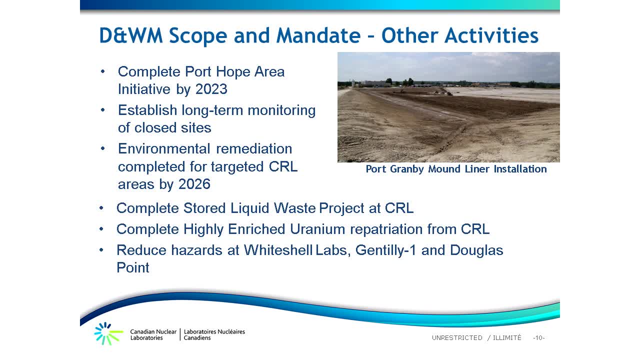 We recognize that accelerating the pace of decommissioning requires that we put in place an integrated strategy for all waste streams. This will start with the new near-surface disposal facility As a permanent solution for low-level and a small amount of short-lived intermediate level waste which meets the safety basis. 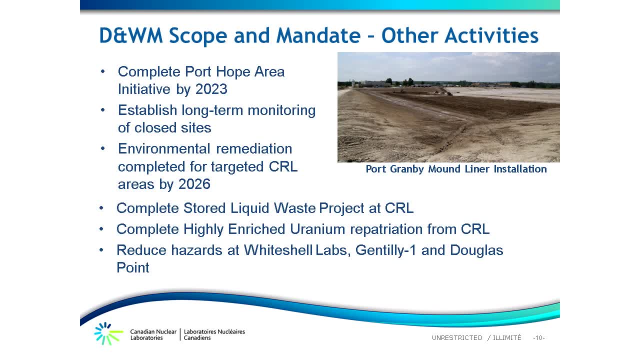 We want to avoid temporary storage solutions and multiple handling of waste if possible. We believe that the optimal approach to decommissioning of the nuclear power demonstration reactor and the white shell WR1 reactor is in situ decommissioning, which will be presented by C&L staff. 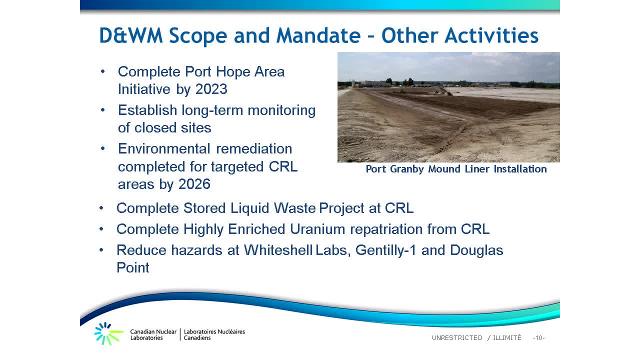 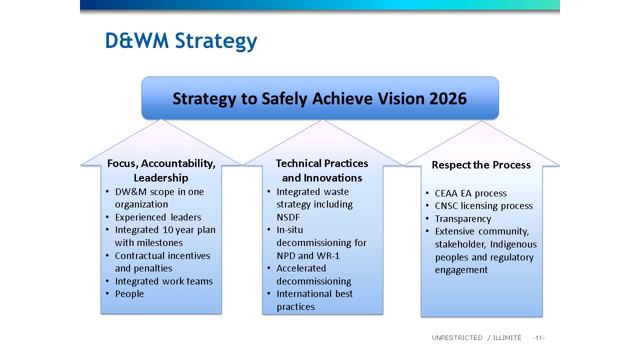 Finally, everything we do is informed by international best practices. In the third element, we want to emphasize how importantly we treat the process. We are confident that our vision represents a safe, technically sound approach to achieve the mandate. However, we understand that none of what we are describing today is predetermined. 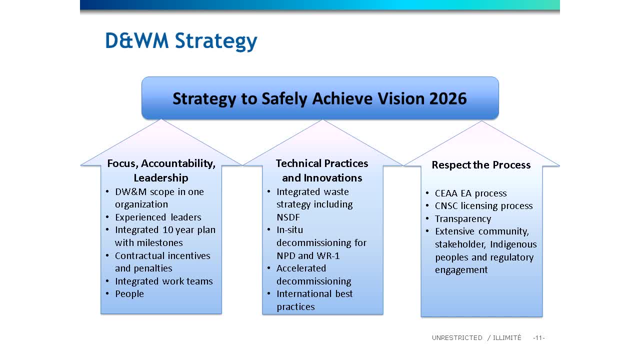 We understand the engagement and need of the community. We understand the engagement and the approvals required. We understand and respect both the environment assessment and the licensing process. We aim to be transparent. We also recognize that we are asking the community and the regulator to absorb. 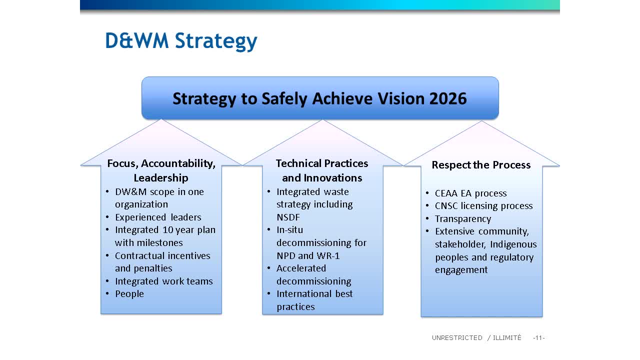 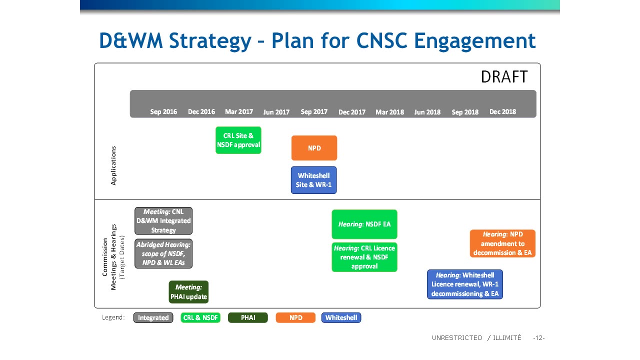 and evaluate a lot of information over a relatively short period of time. We are taking great efforts to make information available and answer any and all questions. This slide demonstrates where rubber is going to hit the road in regulatory space. It shows our planning basis for regulatory submittals and commission appearances over 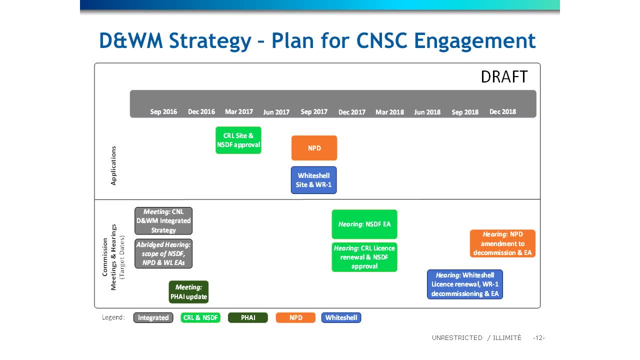 the next 28 months. I want to stress that this is our current planning basis and we recognize that all commission meetings and all hearing dates in the future will be scheduled by the commission. The schedule is aggressive, but we believe it is achievable and we will do our part. 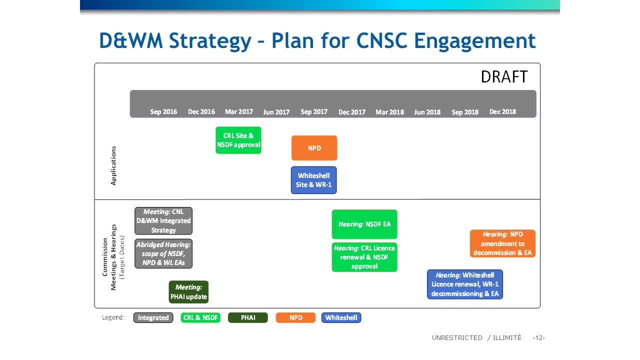 in making complete quality submissions to CNSC on schedule. The slide shows that we will be before the commission many times over the next two and a half years on several different projects, as well as the Chalk River site license, operating license renewal and the Whiteshell decommissioning license renewal. 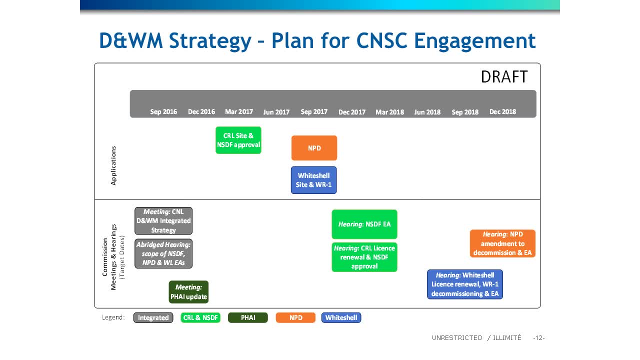 We are taking an integrated approach to the various approvals required. For example, we are coordinating the Near Surface Disposal Facility, environmental assessment and the site relicensing together. We are also coordinating our new approach to the Whiteshell WR1 decommissioning with renewal. 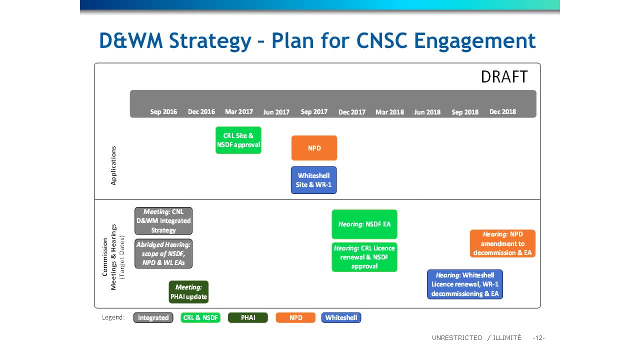 of the Whiteshell decommissioning license Achieving the Schedule 1, we are taking an integrated approach to the various approvals required. This will be a challenge and we are communicating with CNSC staff to ensure we provide submissions that allow adequate time for regulatory review. 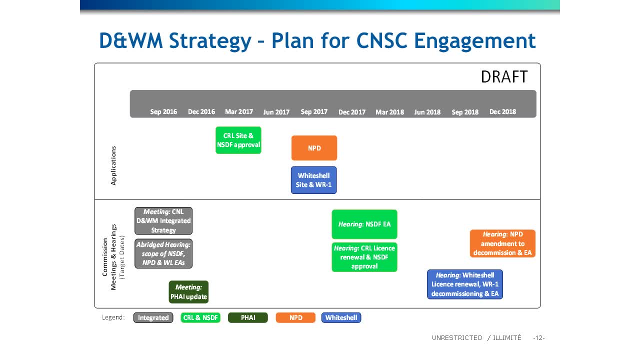 We have an administrative protocol in place for the Near Surface Disposal Facility which is available on the CNSC's website. The protocol lays out the detailed schedule for CNL submissions to CNSC, aligned with the overall schedule for Chalk River site license renewal. 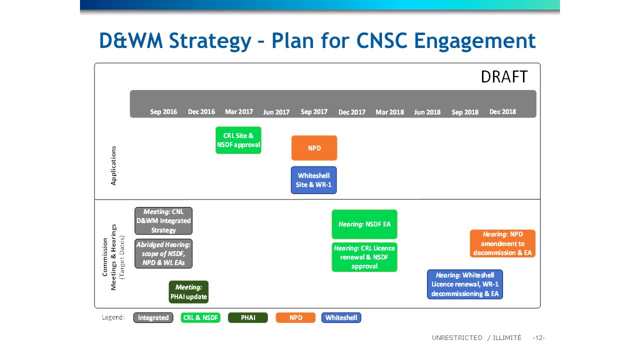 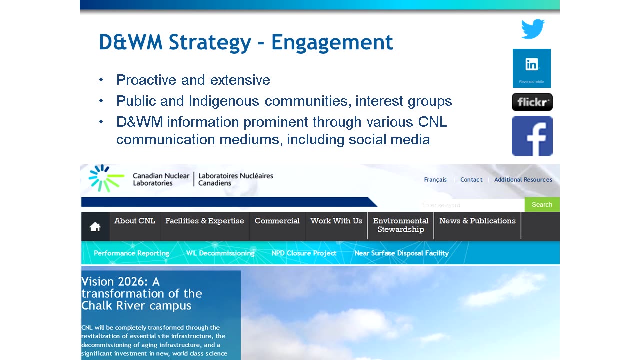 We are developing similar protocols for NPD and WR1,, as they have proven in the past to be effective mechanisms for ensuring the expectations for project deliverables are clearly established and communicated As part of our engagement strategy. this slide shows a partial view of CNL's external home. 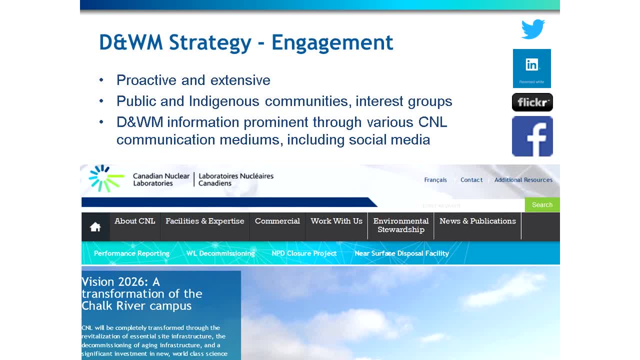 page. The home page is updated regularly, so it may not look exactly like this today. I will use it to illustrate one of several mediums we use as part of our public information program. Prominently displayed on the home page, we have links to the major projects we are discussing. 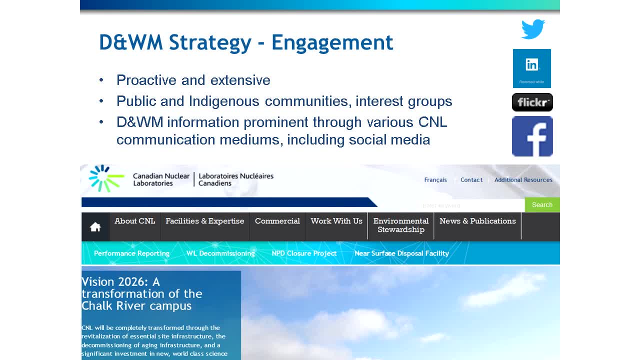 today: Whiteshell decommissioning nuclear power demonstration closure and the Near Surface Disposal Facility. We offer ways through the website for the community to ask questions and to get information on these projects and other CNL activities. We are also active in all well-known social media sites, including Twitter, LinkedIn. 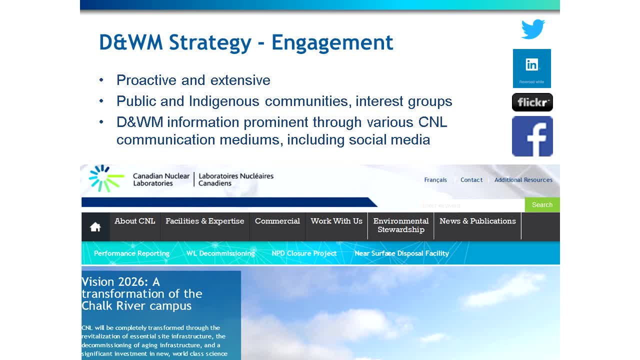 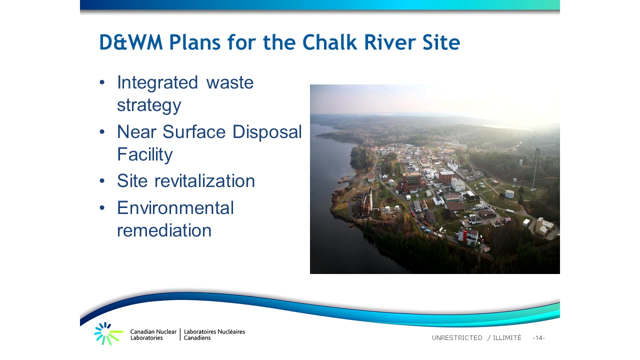 Flickr and Facebook. We are continually looking for ways to engage and address questions on any aspect of our operation. When we talk about specific projects later in this presentation we will provide more specific information on the engagement and the feedback we have received. Having reviewed the big picture view of CNL's scope, mandate and strategy, I'd like to 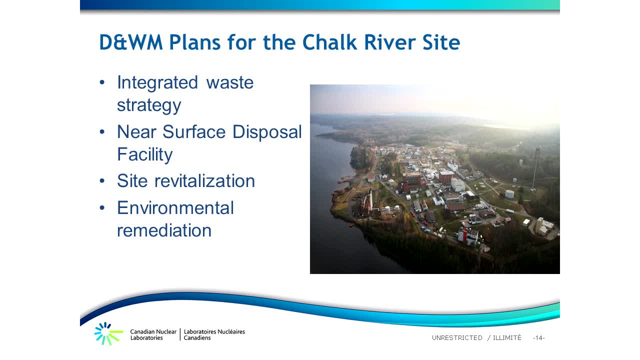 focus for a few minutes on important activities taking place at Chalk River. I'll be covering topics shown on the slide, some of which I've already mentioned, and be parting more depth as part of the understanding. Thank you, Thank you. 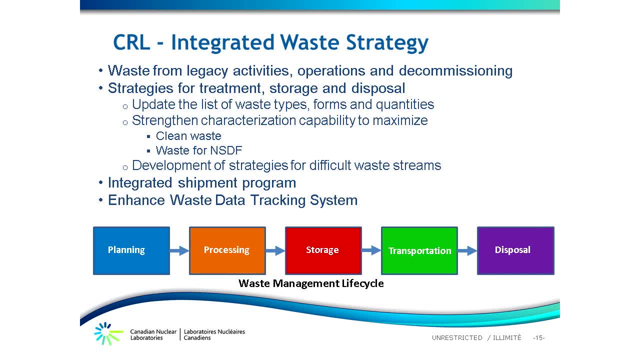 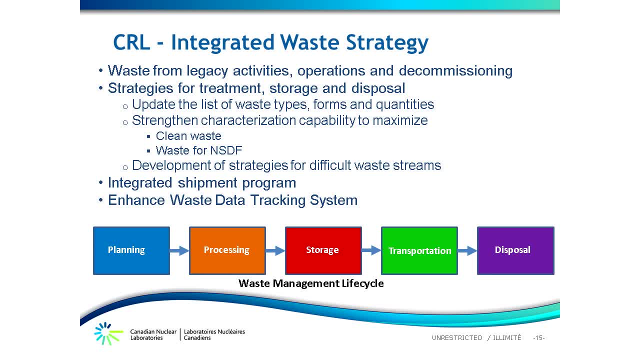 To develop an integrated strategy. we are updating the list of waste types, forms and strengthening our characterization capabilities. this will allow us to maximize the quantity. the quantity of clean waste we can treat as normal industrial waste. for waste that cannot be cleared as clean we want to maximize. 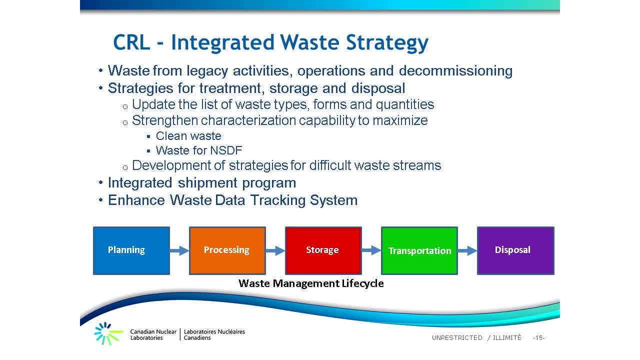 the amount which can go into the near surface disposal facility. the waste acceptance criteria for the near surface disposal facility will be determined from the designs, performance assessment and the safety case as approved in license. other streams will be stored until permanent disposal strategies can be determined. managing all this waste involves a lot of movement and we're 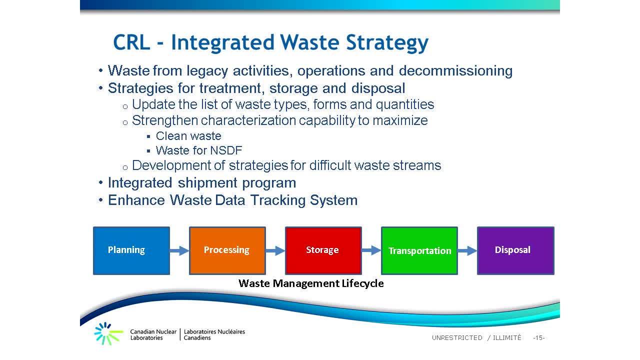 improving our processes to make it more efficient and avoid unnecessarily handling and storage of waste. finally, we're improving our waste data tracking system, which is essential to ensuring we make control of all the waste. development of this integrated strategy is a work in progress, but we felt it was. 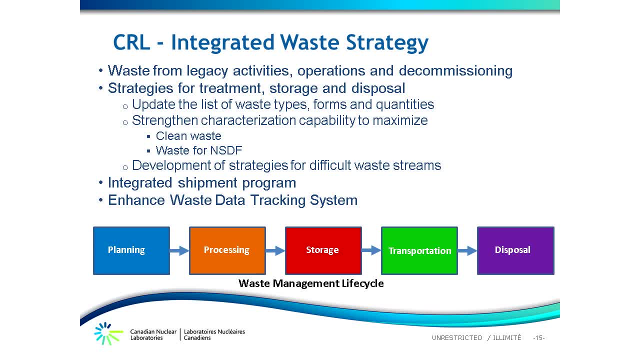 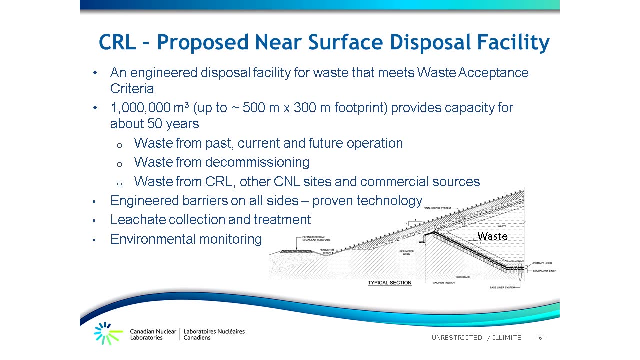 important to let the Commission know we are taking a holistic view of the issue, as we manage the volumes of waste in an efficient and safe manner. the near surface disposal facility that I've already mentioned several times is primarily for waste from past, current and future operations, as well as very 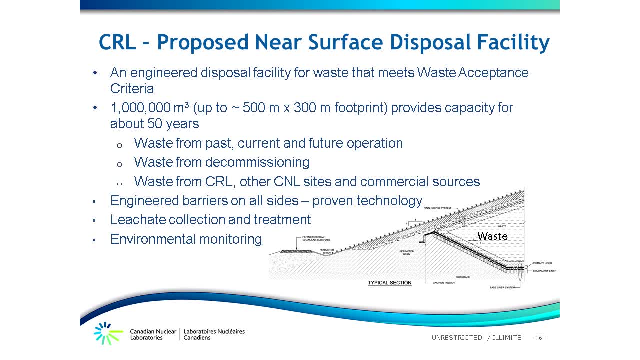 large volumes of waste that will be generated by our decommissioning activities. all the waste adminis admitted to NSDF will meet the predetermined waste acceptance criteria. our goal is to have NSDF operational in 2020. we expect it to receive waste for 50 years. it will 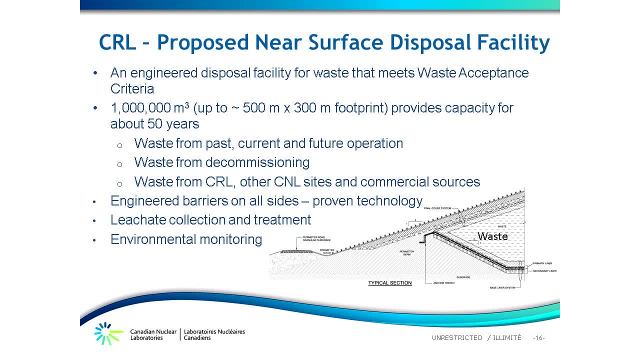 be built in phases with a maximum capacity of about 1 million cubic meters. it is essentially a grade-level facility. as illustrated in the drawing, NSDF will have a large surface area and shallow depth and when covered, it will form a low-height mound that will blend with the surrounding environment in a stiff. 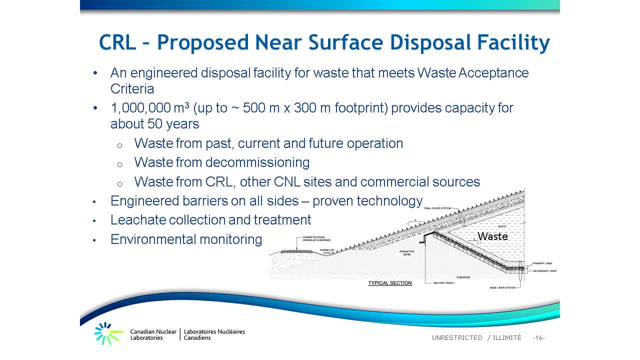 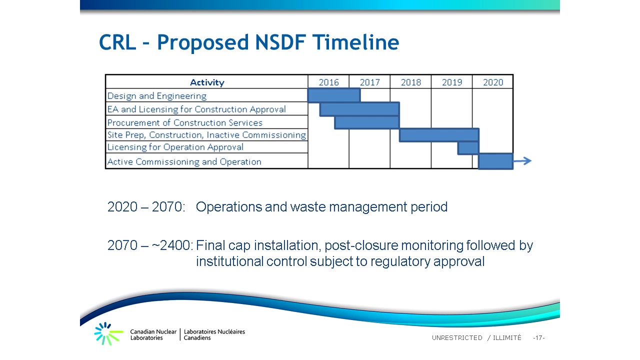 grueling engineered facility that will have custom-designed barriers on all sides, based on proven technology. it will have a leachate collection and treatment facility with extensive groundwater environmental monitoring. this facility will be very similar to the Port Hope initiative long-term waste management facilities. this side slide shows the simplified high-level schedule leading: 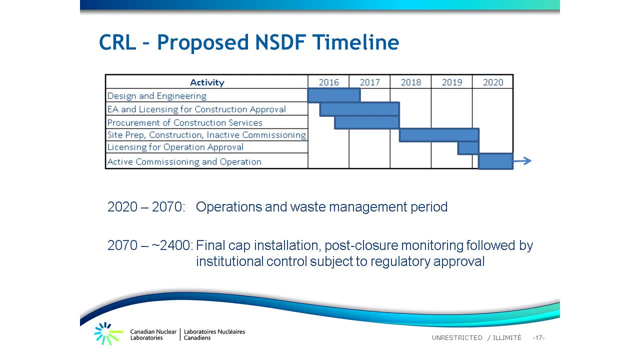 up to active commissioning and start of operation for the near surface disposal facility. we are well into the design and engineering work and the environmental assessment process has started. we are just beginning the process- procurement process- to ensure that we hit the ground running once we obtain regulatory approval. we are planning to receive approval to start construction. 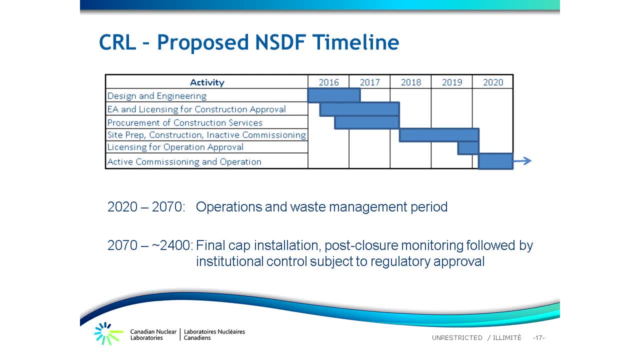 in early 18, with subsequent approval to start operations in early 2020. after NSDF ceases operations in about 2070, there will be a prolonged period of institutional control. the duration of this period is subject to regulatory approval, but we expect it to be on the 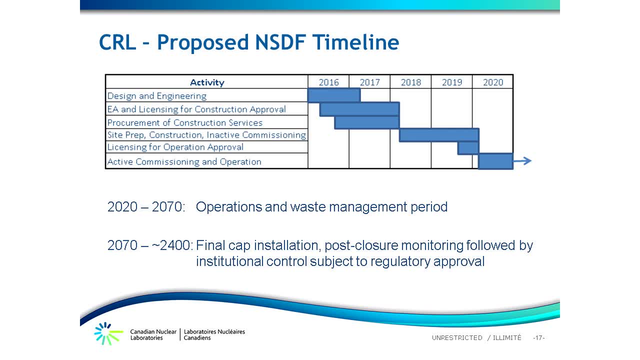 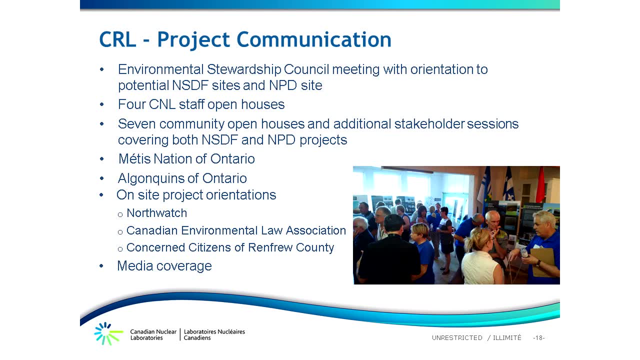 order of 300 years. we are well into the engagement process for the near-surface disposal facility and in many of our engagement activities we include nuclear power demonstration closure project at the same time, given the close proximity of the two projects we are. we still have one final discussion with the National Development and Retail. 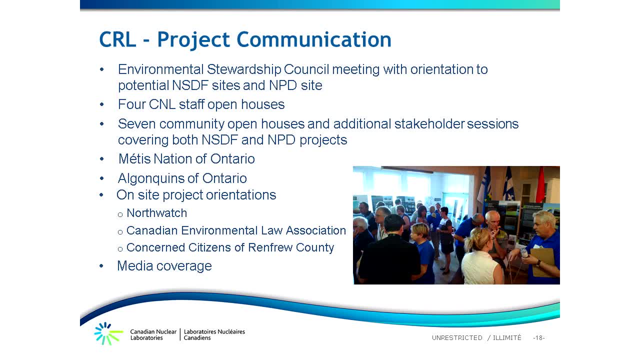 Oklahoma on the national management of our facility. in total, some of the people are troubled and, in push to complete the implementation, we are expecting our molders and theynisse him может have a second around. this talk will focus intよろしくی. thank you forward. seals education. 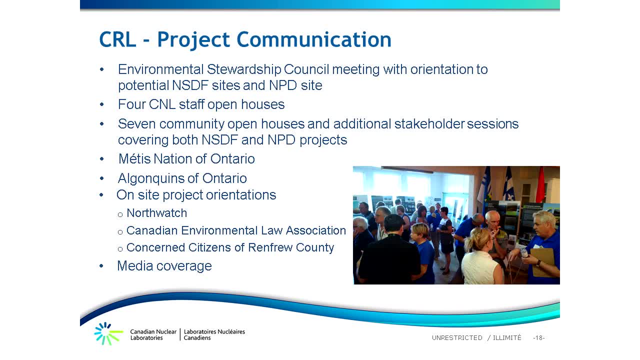 you, I dreaded. I keep saying yeah, that's pretty good, and to hand over the next session. we will shift back to the district service and the city staff writers and leaders to guide our leadership and Contractors in Laurence. best of all the to keep in touch with everyone in Open House and Regional Restoration in the. 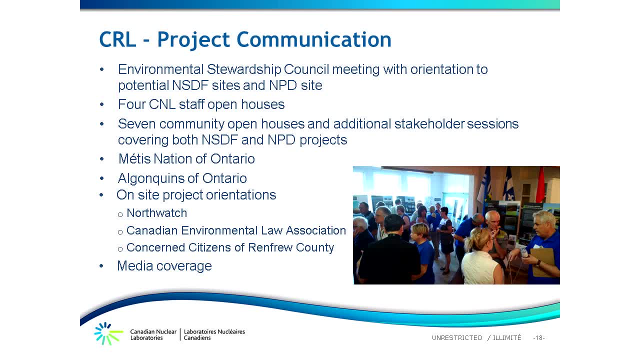 area. give Thanks to Isaac- one of our history- individual leaders andchenly pitchers and actively informing those we need to know, those we know are interested in the community at large. when we have new information, there is a definitely an interest in our projects and we welcome the engagement. further engagement. 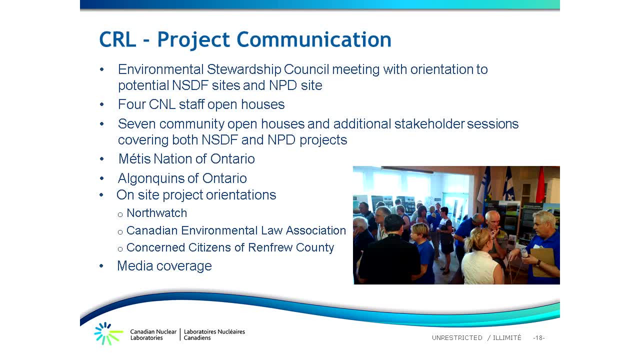 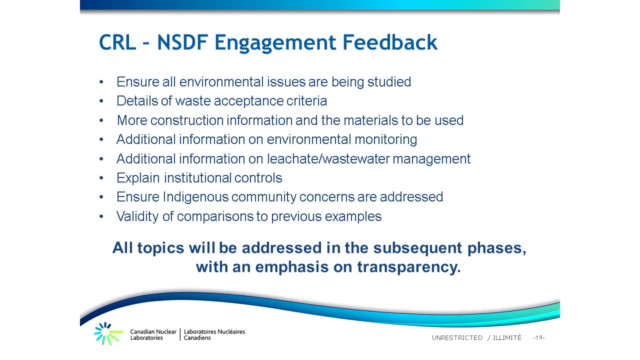 activities are scheduled for this fall, actually starting next month, and throughout both the NSDF and NPD closure project schedules. this slide shows some of what we heard, some of what we have heard from engagement activities. there has been positive feedback, encouragement that we are taking action to reduce hazards in a permanent way. as you can see, a number of 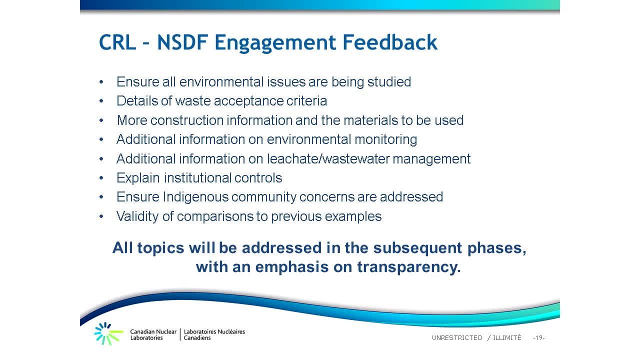 questions and issues have been raised and we take them all seriously. where we were not able to provide immediate responses to questions, we will address the feedback in subsequent phases of the project. primarily you. this slide shows some of what we have heard from the NSDF and NPD. 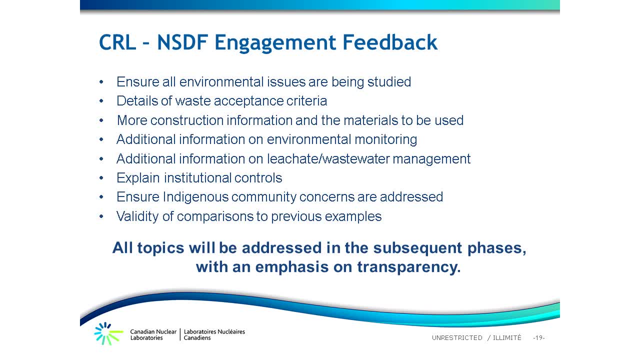 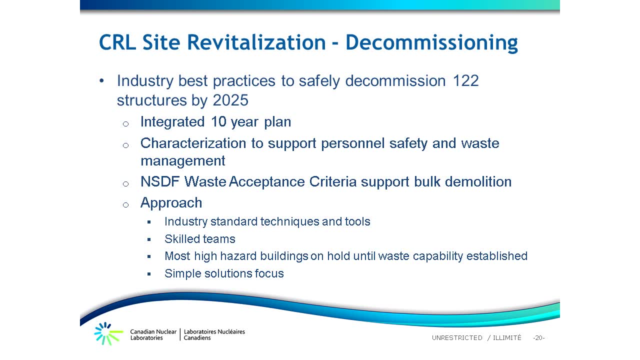 and we are taking action to reduce hazards in a permanent way. as you can see, we are taking action to reduce hazards in a permanent way. as you can see, we are taking action to reduce hazards in a permanent way. as you can see, one of the main waste streams for the near-surface disposal facility is the. 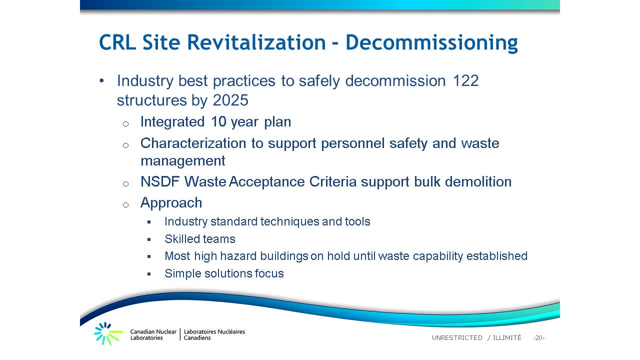 waste from decommissioning 122 buildings at Chalk River, which is one of the most critical steps for site revitalization. to support that characterization is key to the future of knowing what the Waste Are in where to take them. our intention is that the waste acceptance criteria will support both both demolition approach, so we can. 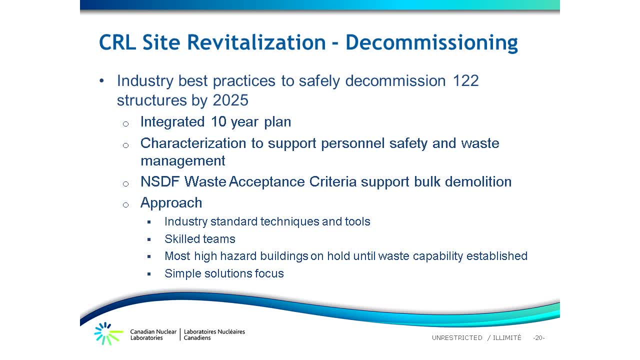 efficiently demolish many buildings and move waste directly into the near surface disposal facility. this is to avoid interim storage, additional handling and most, but as part of this, most of the contaminated facilities will wait for demolition until the near-surface disposal facility- american" near-surface disposal facility- is available. and finally, we will look for. 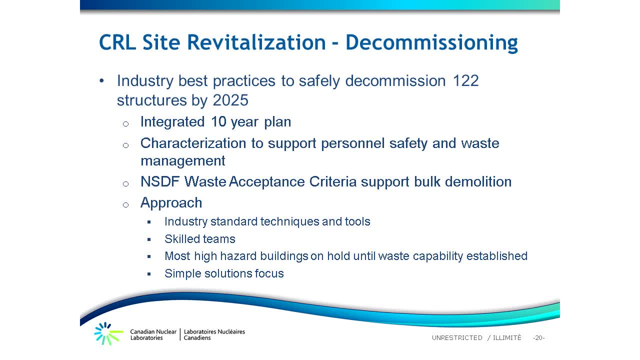 simple solutions that are safe and cost-effective. we'll apply a risk informed graded approach, fully keeping with CNSC requirements. this will allow us to apply techniques that are appropriate for the type of hazard, resulting in cost-effective and safety commissioning. our decommissioning work at CRL has already commenced. I am pleased to report that, since we arrived, 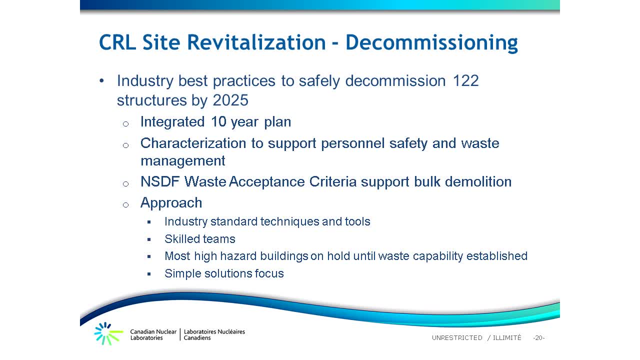 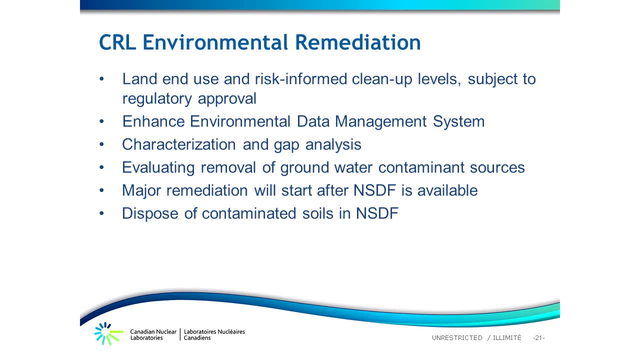 a year ago. we have safely decommissioned and removed 19 buildings with no lost time accidents. the final slide of this selection of this section of the presentation addresses environmental remediation at the Chalk River site. our plans are under development but we are working on accelerated remediation and 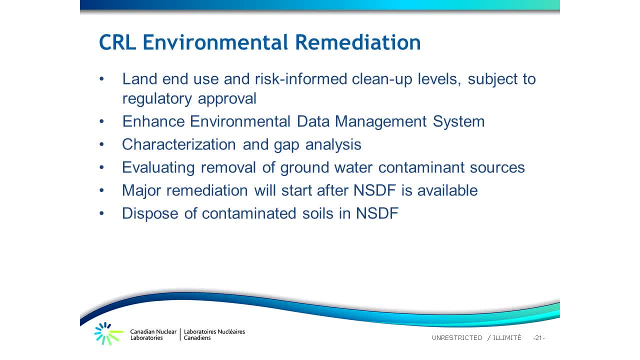 cleanup of the overall site. first we need to establish clarity on the cleanup criteria and intended future use. this will inform the risk informed cleanup levels required for the future. we will enhance the environmental environmental data management system so that we can better understand and analyze the environmental status and 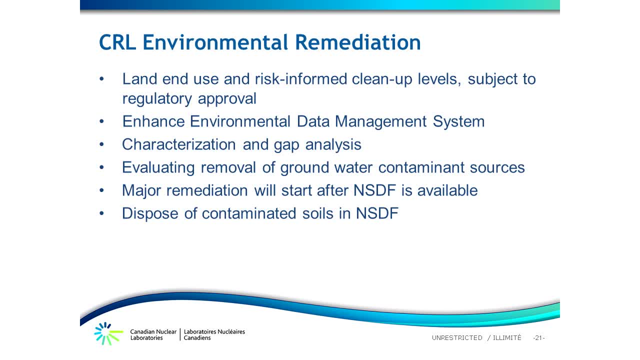 impact of our activities. this will support improved characterization and will all allow us to identify gaps to some needed support remediation decisions. importantly, we are commencing evaluations to remove sources of groundwater contamination. the Commission will recall that, and the underground plumes at Chalk River are a source of discussion at every license. 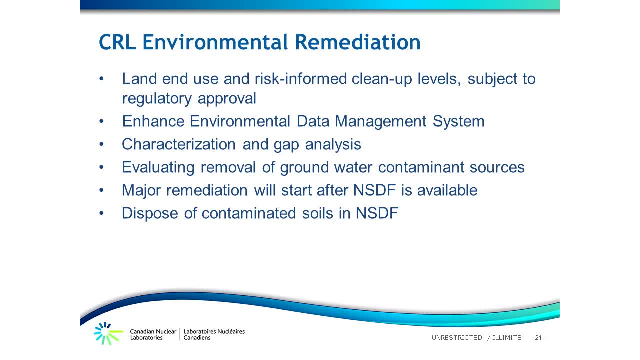 renewal and sometimes in between. if it is feasible and makes sense to eliminate the source an accelerated fashion, we will do so. in terms of the timing of major remediation at the Chalk River site, it cannot start in a big way until waste disposal is available and you're. 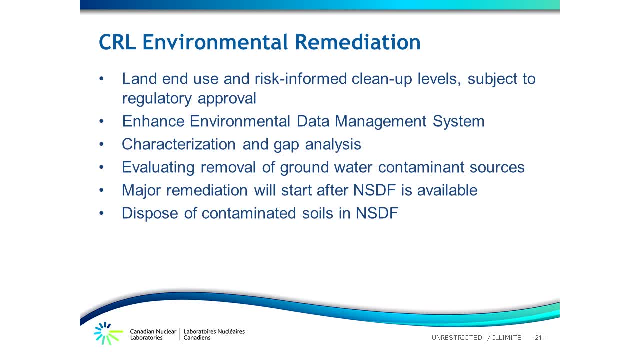 probably aware by now how important the near surface disposal facility is for this all these activities to come together. the final point here is that we intend to use the low level contaminated soils at the Chalk River site for much of the fill at the nurse near surface disposal facility. this fulfills two. 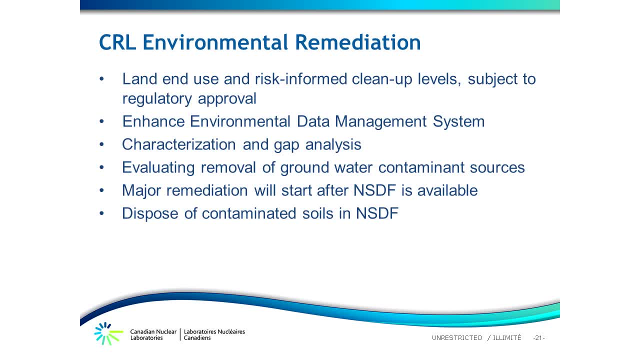 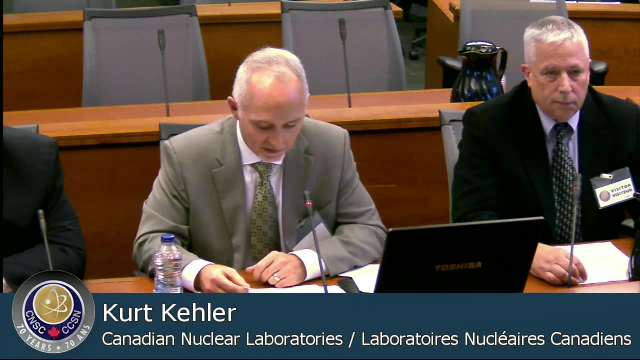 important purposes. first, it provides the bulk internal structure and the drain to the Chalk River site for building debris in the landfill and second, it means we only have to clean it and move material. once this includes this part of the presentation, I'll ask now: ask Pat Daly to go through the NPD closure project presentation. Thank You, 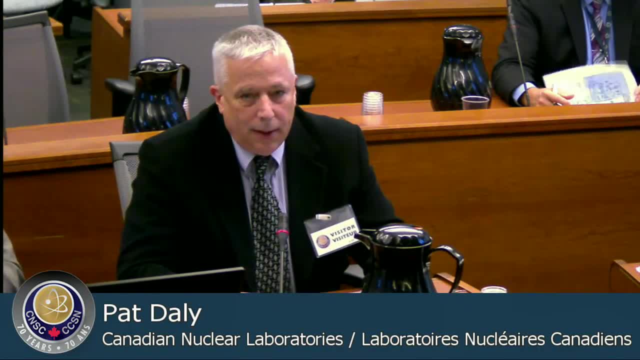 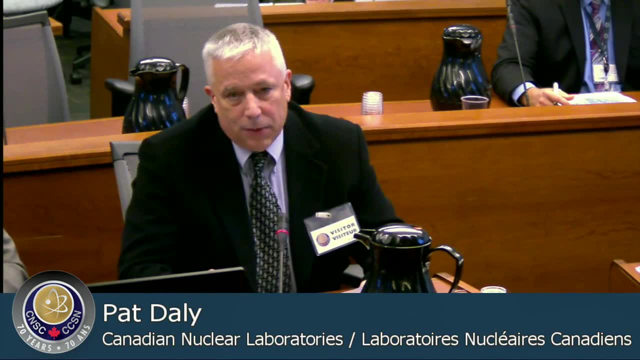 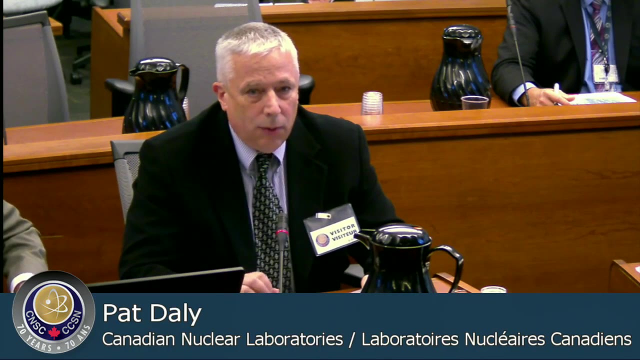 Kurt, good afternoon. my name is Patrick Daly. I have responsibility for the NPD or nuclear power demonstration closure project. during this presentation I'll go through our strategy, our plans and our approach for that closure. NPD was the first can-do reactor and it was the first prototype reactor to demonstrate. 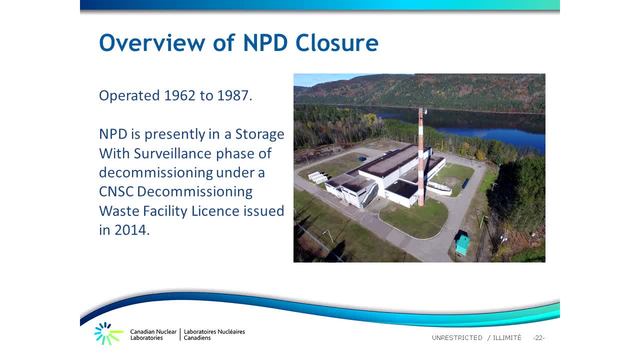 nuclear electrical power generation in Canada. the current- the current photo that you see on a slide there. that is the current configuration of the plan at this time operated. operated from 1962 to 1987 when it shut down. there were numerous other buildings on site, including training facilities, administration. 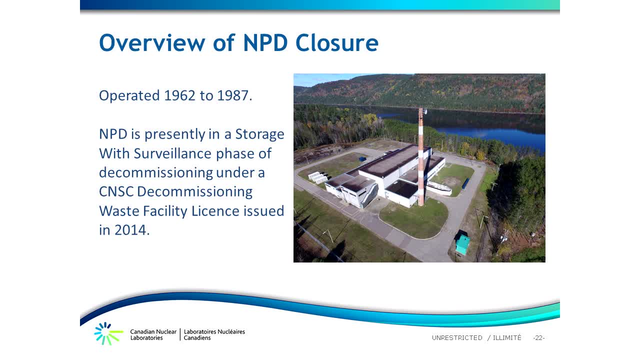 facilities. those have all been removed shortly after the they shut down in 87. in addition, much of the above-grade equipment was removed from inside the building, for example on the commonly referred to as the secondary side of the plant, the condenser, the turbine generator, the control room. all those 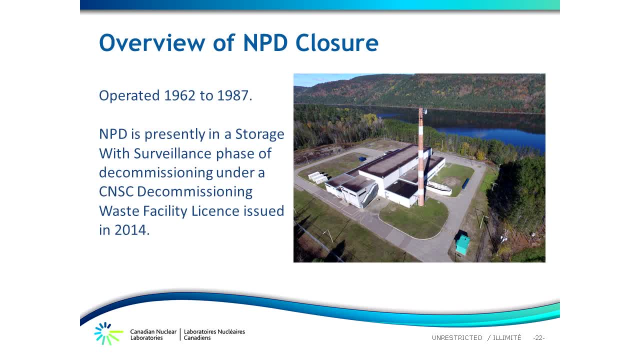 things are gone, but what is left is what is below grade amp. ed is currently under storage with surveillance and it has a decommissioning license. as we go through our closure project, safety of both employees and the public will be the overriding priority for the project, followed by an including Environmental. one thing I would point: 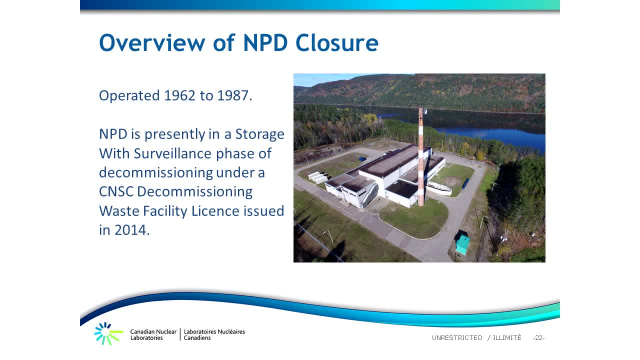 out on that photograph is the ventilation stack, which is a prominent feature right in the middle. that is a very important part of our project. it does impact a species at risk and I'll go into more details a little bit. following shutdown in 1987, MPD was defueled. all fuel is removed from the 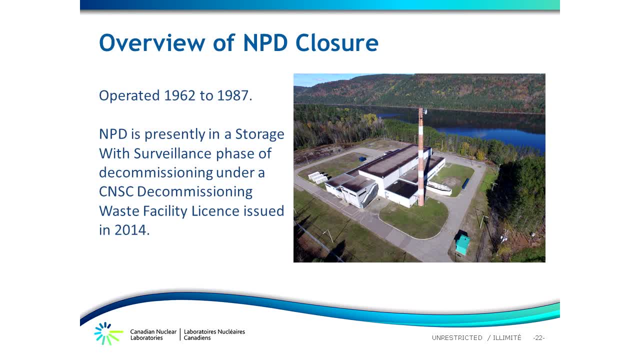 site and is stored at Chalk River at this time. in addition, all the systems were deactivated, the heavy water was drained, the systems were flushed and dried and then there is no, no heavy water, no light water, and again, all the systems have been deactivated at the site. the radiological hazards that 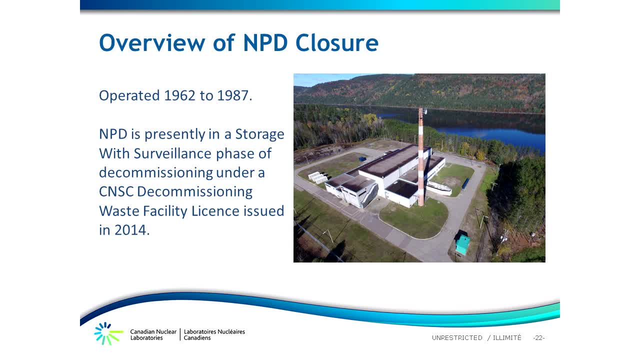 remain are principally the hazards associated with activation products with the reactor and in the biological shield around the reactor, and then contamination- residual contamination and the heat transport system, like in the boiler room and the fuel bay. if you looking at the slide there, six, five and four represent the area that is actually in a containment: reinforced concrete. 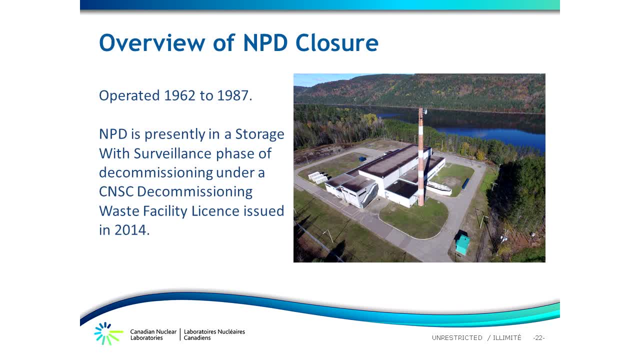 containment below grade. six is the fuel bay, five is the reactor bay with the calandria, and then four is the boiler room. the other blue portion on the slide is a condenser bay. all the equipment from that area has been removed and then the above grade. 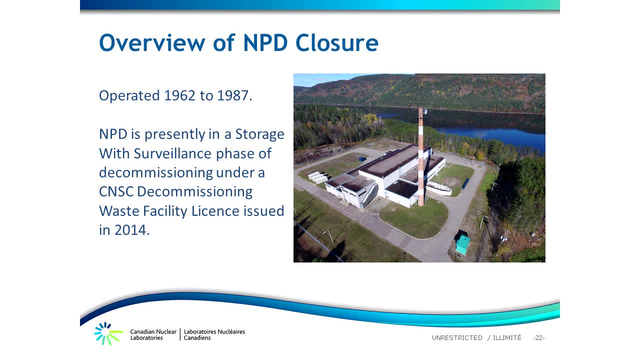 structures represented as one, two and three. when we finish closure, those structures will be removed and the bulk of that debris will be placed into condenser bay for MPD. our approach, our preferred approach- and we'll go more in detail- is to take the lower containment structure with all the intact reactor. 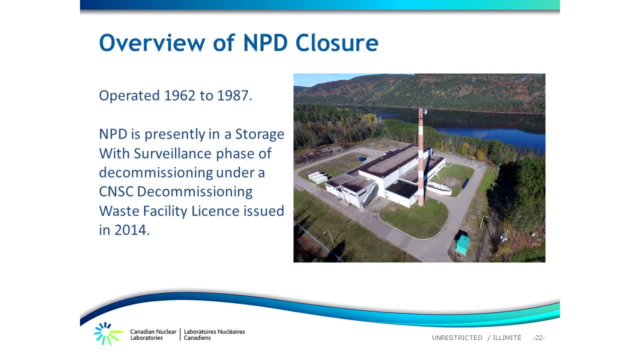 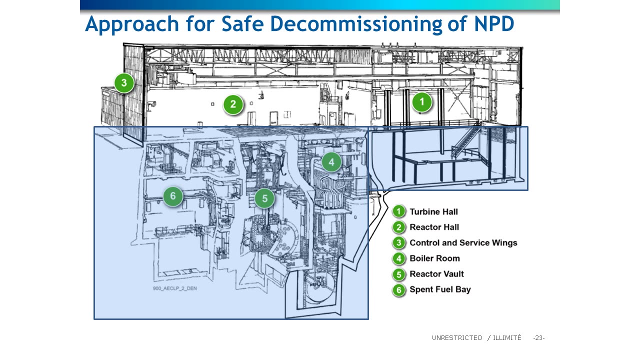 systems and equipment and entombment and we call it in situ decommissioning. but it will be grouted in place with a reinforced concrete cap and then engineered clay cap on top of that to disperse water. CNL will be applying to CNSC for an amendment to its license to a. 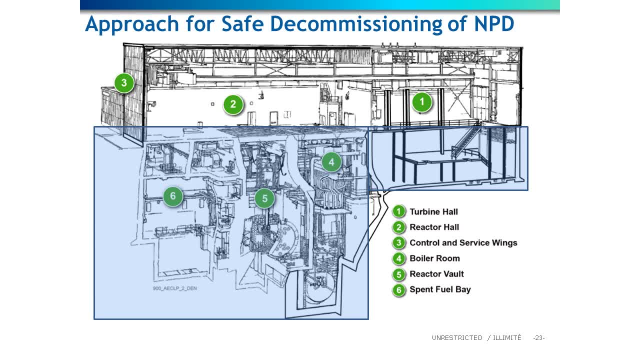 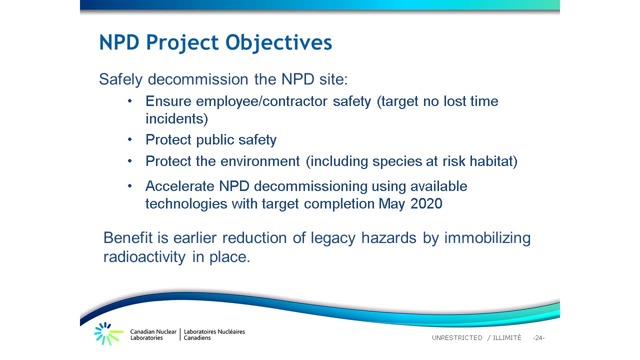 new would be required by the CNSC: safety. safety is our number one priority. we've we firmly believe that if our employees don't get hurt, the public is not in danger of being hurt. so it's it's. we focus on our employees, we focus on the public, and then we can get the plan that's going to help us do this all right. so first we'll look at the 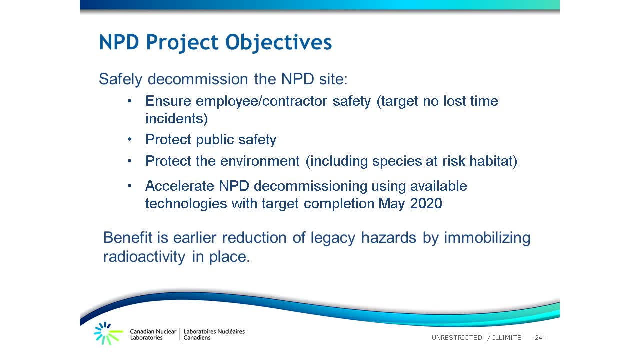 Then finally, the environmental impact. just a little bit of background on MPD. There's approximately 1,000 acres. MPD is located about 30 kilometers northwest of Chalk on the Ottawa River. There's approximately 1,000 acres at the site. Of those 1,000 acres, there was 25 acres impacted by construction and currently there's about six acres that are under license. So it's a very small footprint that's been impacted and, within that area, that's going to be impacted by our closure process. 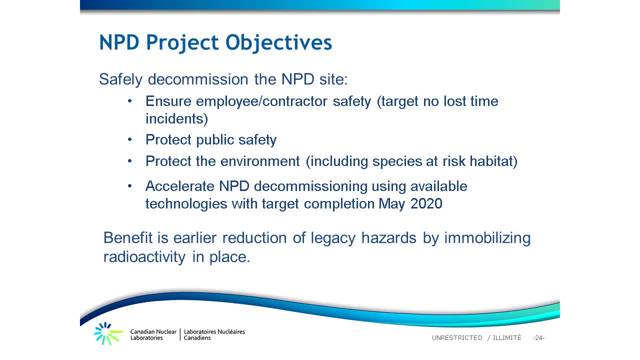 the ventilation stack is an area where there is a species at risk. Our original plans were to design and build an alternate habitat and then remove the stack. after engaging with stakeholders, regulators, including Environment Canada, We've decided the best way to do that is to remove the stack. 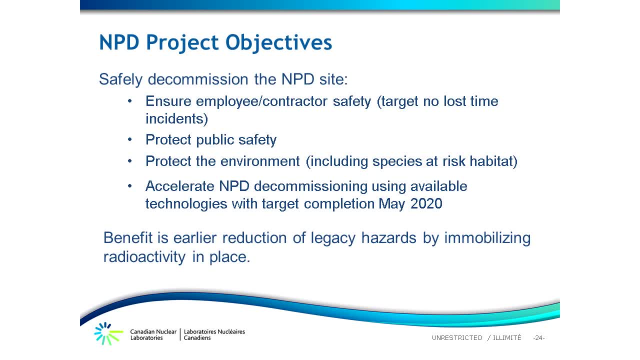 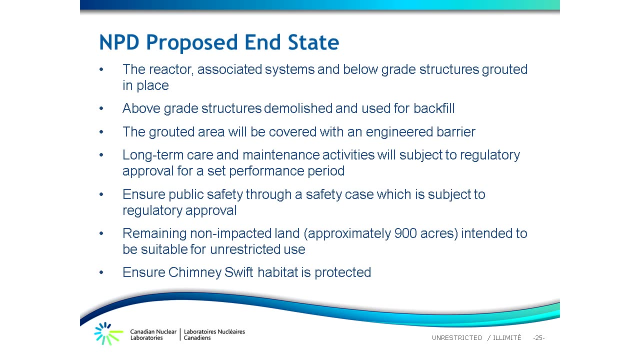 and the best approach is to leave the stack. So we have analyzed the stack and when we're done, the stack will remain to support a roost for the chimney swifts in the future. going forward Again, our tentative schedule right now: overall duration: 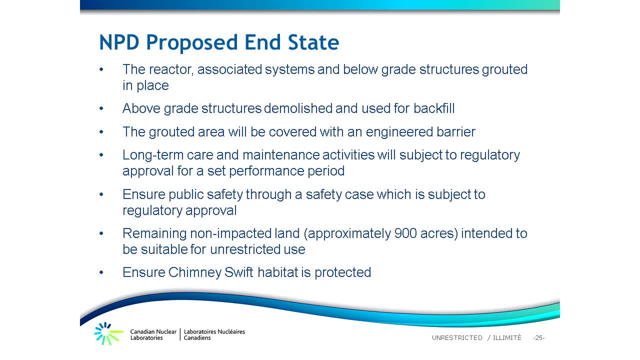 we're looking to have final closure by May of 2020 as our target. The proposed end state is, as I mentioned on that previous slide- is to have all the reactor systems within that reinforced concrete containment grouted in place to encapsulate the systems. 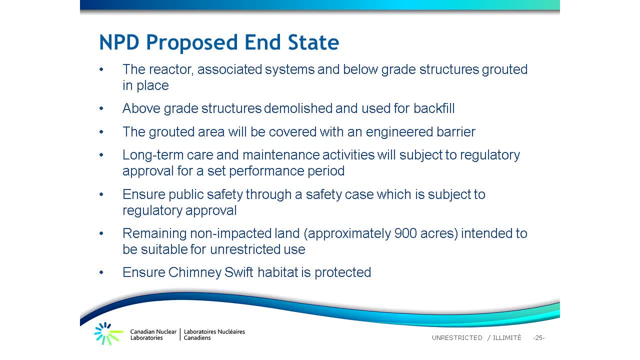 and demolish the above-grade structures Right now, then we would install a reinforced concrete cap and an engineered clay cap on top of that to disperse any surface water away from the entombment, and we believe this will offer the most, the most robust long-term final state for NPD. 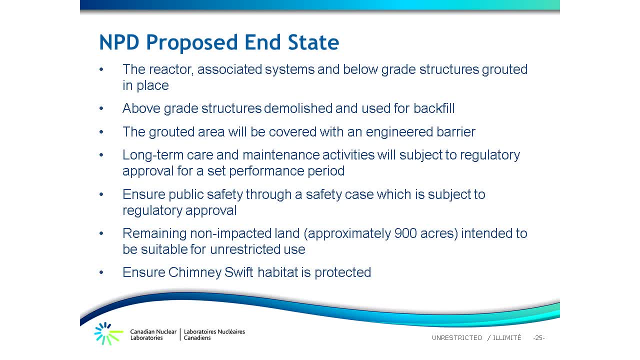 So it will become a near-surface disposal facility in itself. when we're finished, This will be an equivalent of one. We have no intention of bringing anything into NPD. It's only what exists there now- below-grade- that will be entombed. 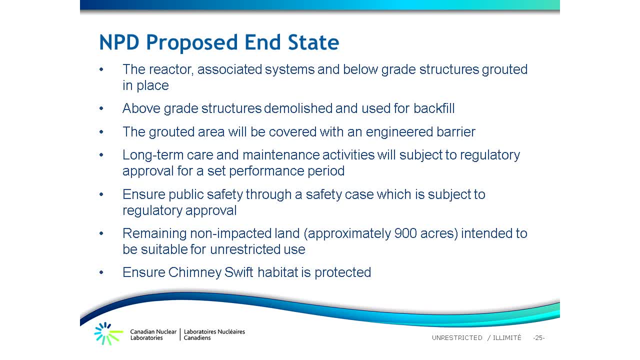 Nothing else will be brought in. As I mentioned about the footprint, the actual footprint of just the entombment area is about 150 meters by 50 meters. That's the square footage if you're looking down on top of it. When we're finished, we've amended the license. 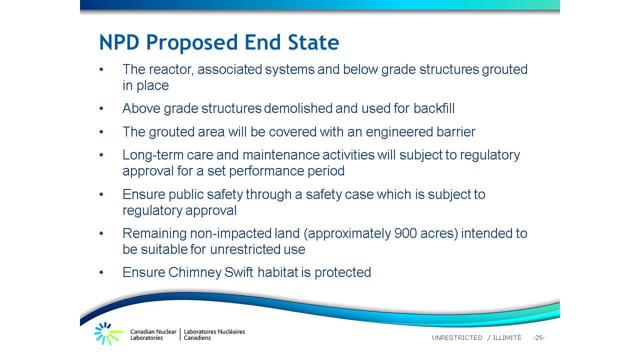 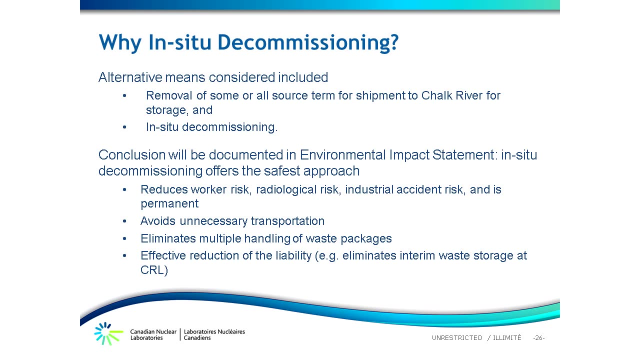 Approximately 950 acres will be available for other uses and be returned to ACL for consideration for future use, for whatever use they deem appropriate. As I mentioned, the ventilation stack will remain for the chimney swifts As we go through our process with the environmental 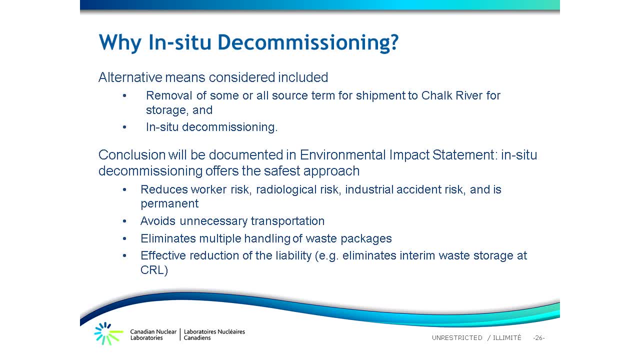 environmental assessment, we have looked at alternatives. What I've described to you is our preferred alternative. The other alternative is a partial removal, a source term or removal of everything below-grade. In doing that, it would mean packaging, transport to chalk for interim storage. 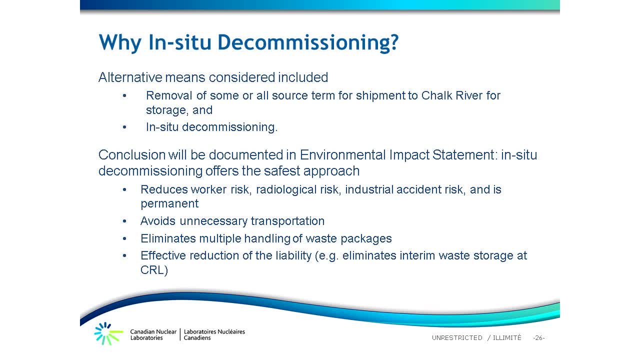 and then eventually, at some point when permanent disposal is available, it would be disposed of at chalk. Those are the alternatives. We believe our approach is not only to the most robust approach, given the fact it already is contained within a reinforced concrete containment. 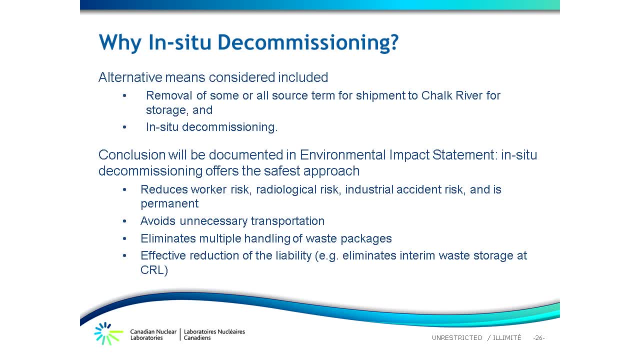 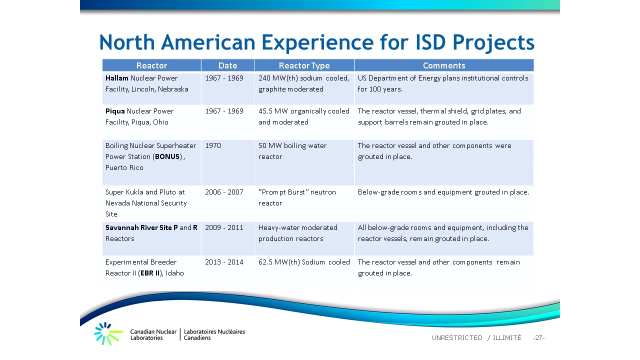 but it also minimizes exposure to employees, both from an industrial safety, industrial hygiene and from an ALARA point of view, as well as eliminates unnecessary transportation of waste on public highways and multiple handling of waste. at the Chalk River site, There have been a number of reactors. 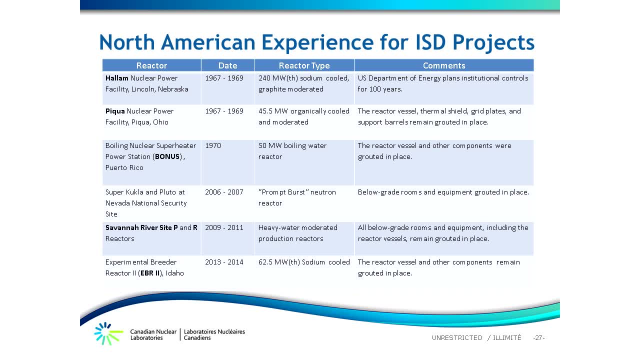 that have gone through in-situ decommissioning or entombment within North America. There were three reactors that were entombed back approximately 45 to 50 years ago. These were small test and research reactors. The institutional controls placed on them. 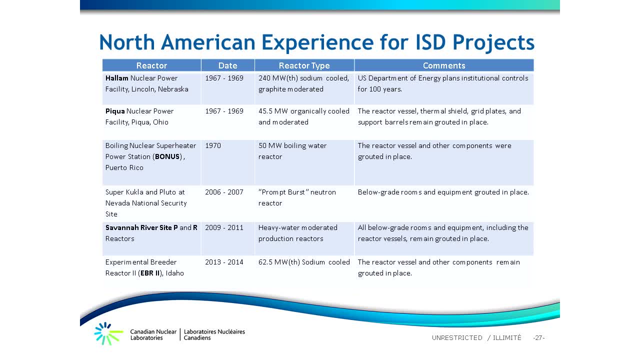 involved periodic monitoring of groundwater and to date nothing has been detected of migrating out of any of these facilities at that time. The most recent experience has been at Savannah River. The Savannah River has entombed two production reactors, and also up in Idaho. 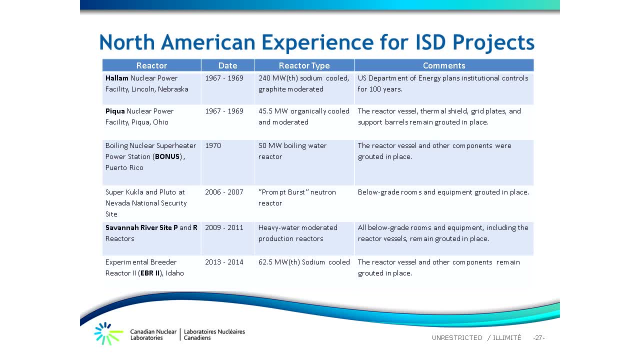 the experimental breeder reactor 2 was entombed up there as well, using a grout approach where they grouted everything It was below grade grouted in place. We have engaged with subject matter experts from Savannah River National Park in the lab who have done a lot of technical work. 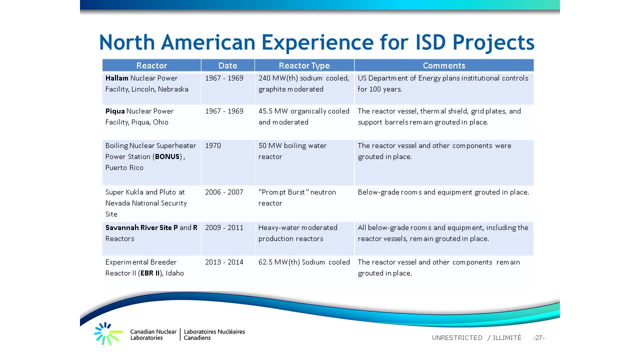 on grout formulas, grout placement. They are going to support us, as well as they're going to support Dan over at WR1, in helping us develop those formulas, as well as help us in our pathway analysis and final closure analysis. The next slide is just a high-level schedule. 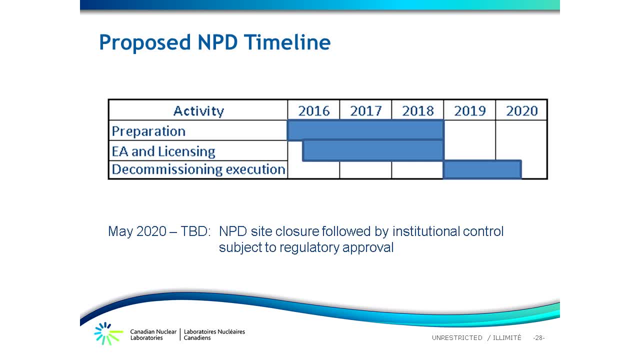 We're currently in our preparatory phase. We do have we have contractors in place for helping pulling together our environmental impact statement, our licensing plan. We do have we pulled together this year our historical site assessment. We also have our characterization plan. 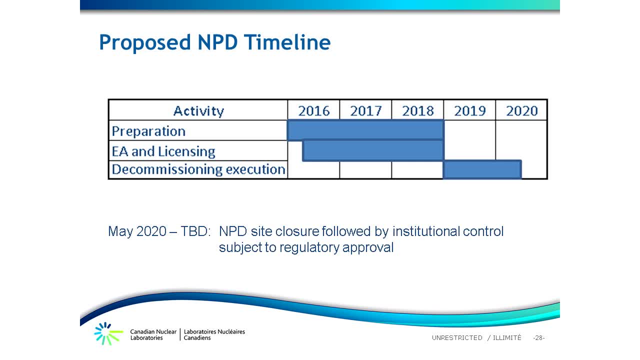 We're doing some work inside the facility to ensure that we can place individuals back into the facility safely, because the facility really nobody's worked in the facility for 30 years. We put them back into the facility safely so they can do the final characterization. 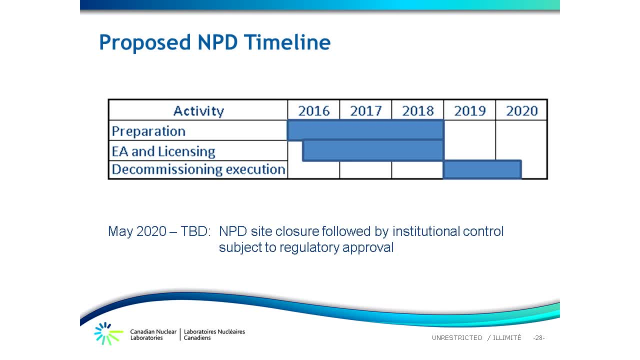 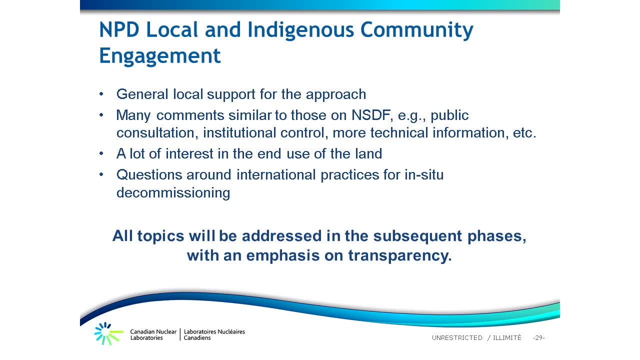 and sampling inside the building. that again will support our licensed submittals. The final once we our intent is to have all the submittals into the staff CNSC staff by the fall of 2017.. That would include our environmental impact statement. 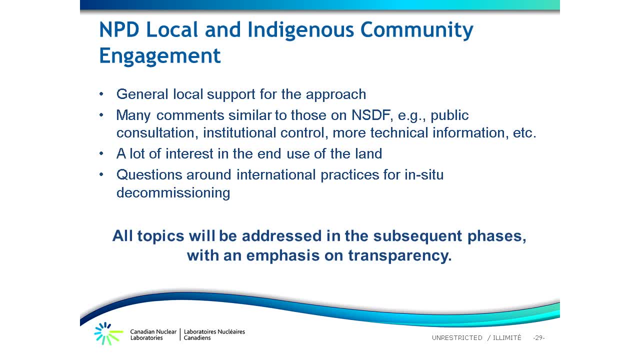 our updated safety analysis and our detailed decommissioning plan And then we hope to, by the end of 2018, be able to move forward to go into execution phase, which then would be the grouting, demolition and final capping of the site. 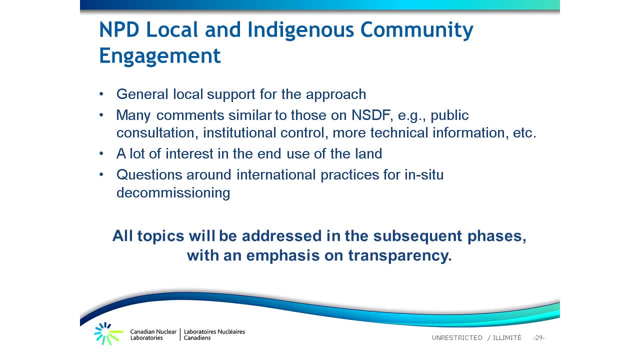 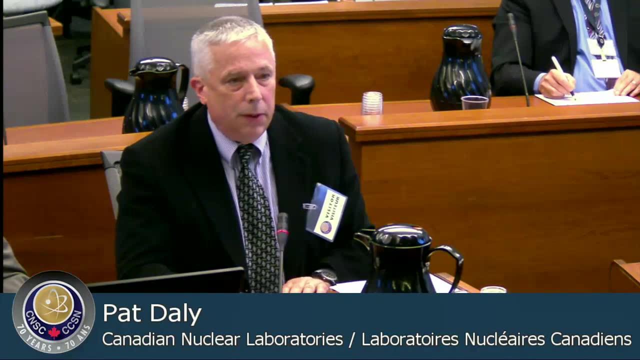 And we estimate that would take about 12 to 14 months to do that, to reach final closure, And then it would go into a period of institutional controls. With that, I was going to turn it over now to Dan Coyne to talk about the white shell. 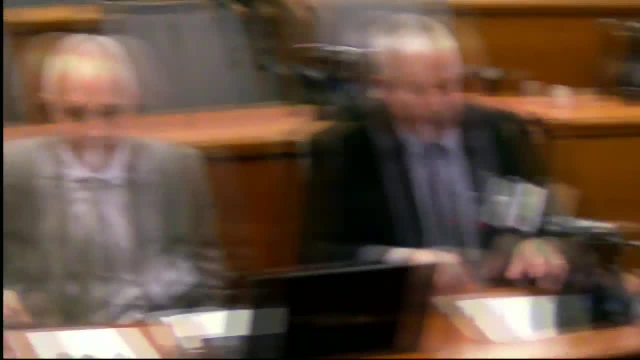 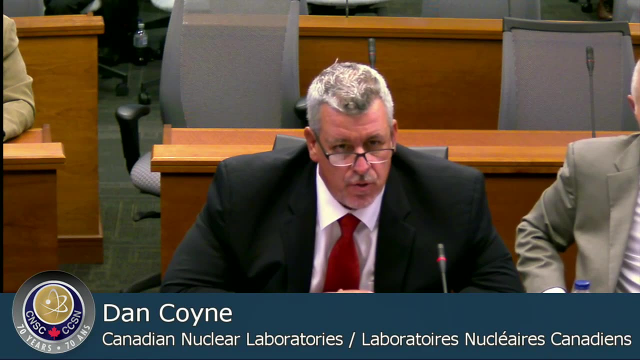 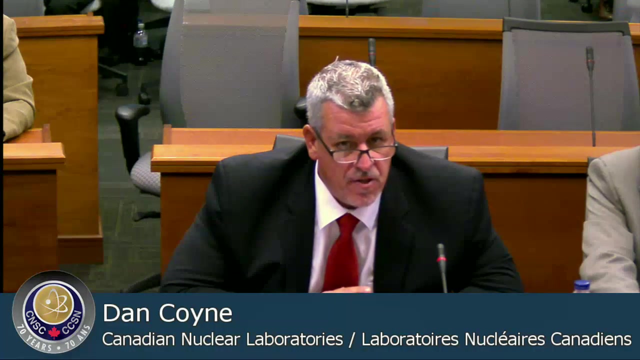 Thank you. Thank you, Pat, Good afternoon. My name's Dan Coyne. I'm the general manager of the White Shell Laboratories Closure Project. I'm going to, in these next few slides, I'm going to describe our strategy and plans for decommissioning. 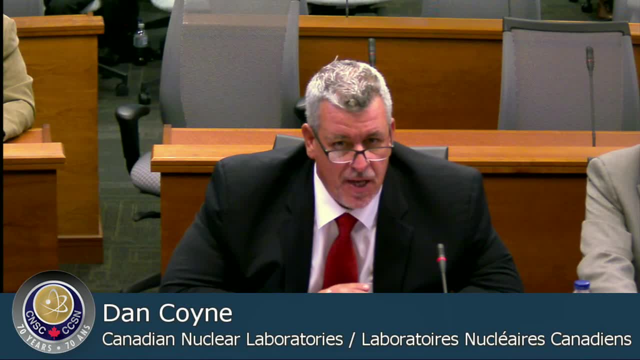 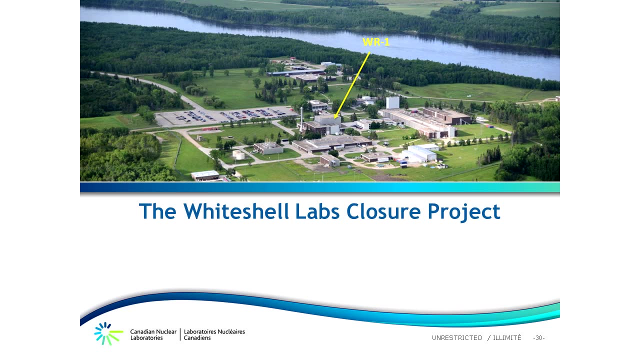 both the white shell reactor and progress and plans on decommissioning the white shell site. The picture on this slide shows the main campus of the white shell laboratory site As it was prior to September of last year, with WR1 reactor building noted in the middle. 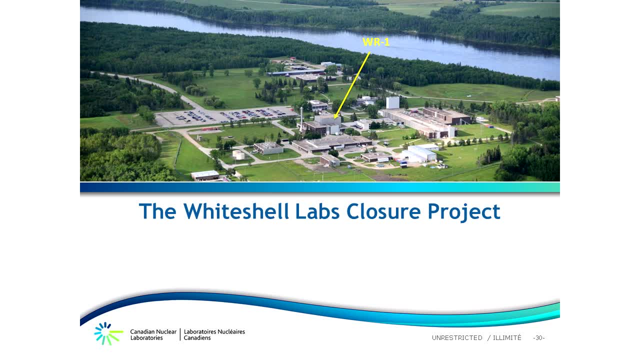 WR1 was a research reactor that operated from 1965 to 1985.. The reactor is presently in a storage with surveillance under the white shell site decommissioning license that's valid to 2018.. We propose to decommission the WR1 reactor. 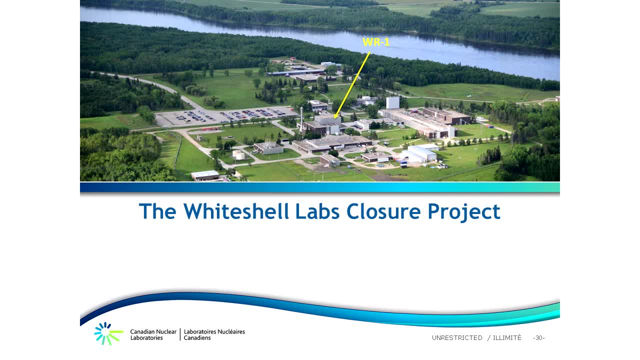 in accelerated schedule. WR1 was a research reactor that used organic coolant. After its final shutdown, the WR1 reactor was defueled and all the fuel has been transferred on site into safe storage at the waste management area at white shell. The heavy water and heat transport systems. 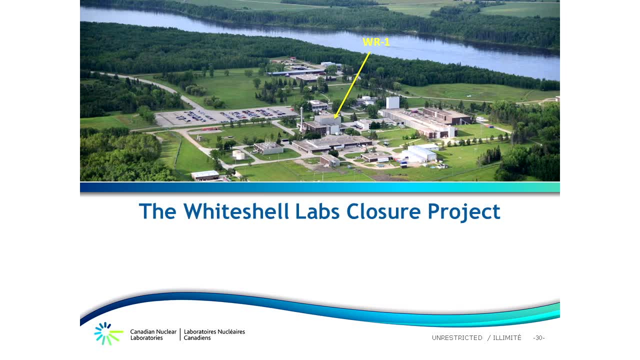 were drained. The remaining hazards are mostly components that have been activated and there is some residual contamination inside of the heat, transport and auxiliary systems. I want to reemphasize that we're going to conduct all decommissioning work at white shell with safety as the overarching priority. 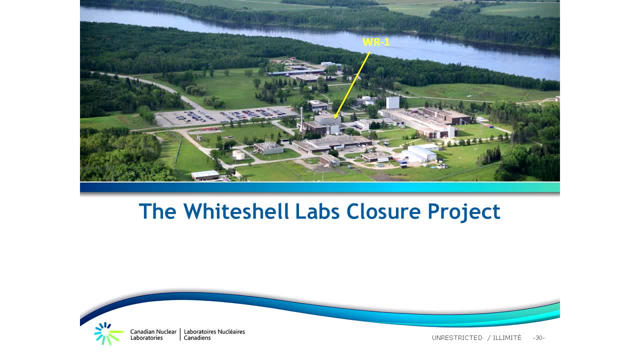 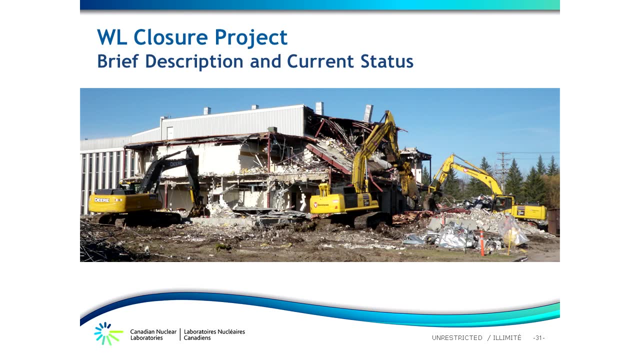 Our motto is: if it can't be done safely, it won't be done. This slide shows the early progress on building 300, phases four and seven. Building 300 is a former analytical lab facility at white shell. The demolition is now complete. 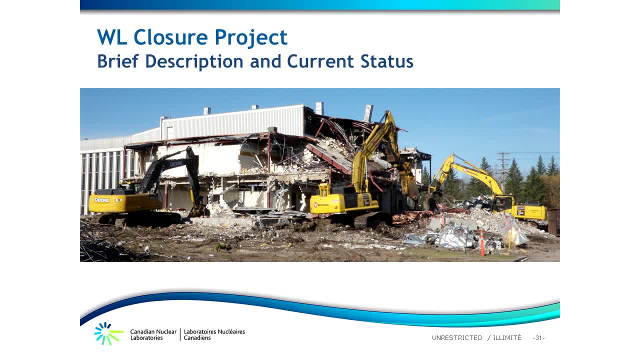 It was the first demolition of a former nuclear mission building at white shell. The slide illustrates a good example of the demolition approach we are following at white shell, which is quite simple: involves heavy machinery to quickly, efficiently and safely demolish buildings like the one shown in the photograph. 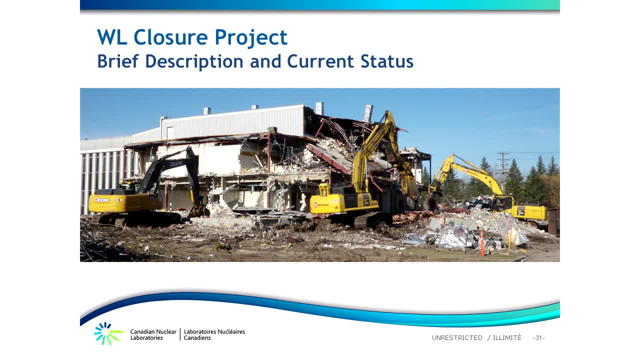 The more laborious part of decommissioning involves the removal of facility systems, components, decontamination and final survey prior to demolition, which all happened prior to our assuming the contract and after we got the contract last September, In April of this year. 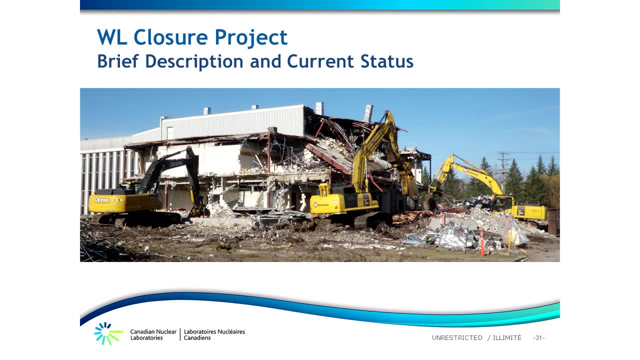 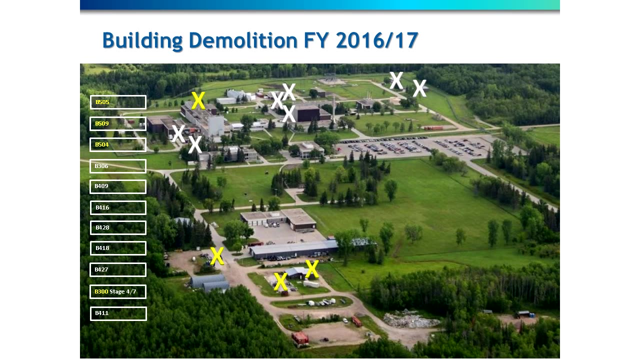 the commission received a comprehensive update on the status of the decommissioning of the white shell site. Therefore, I will focus on progress since then and our plans for the remainder of 2016-2017.. This slide provides a visual representation of the 11 buildings scheduled for demolition. 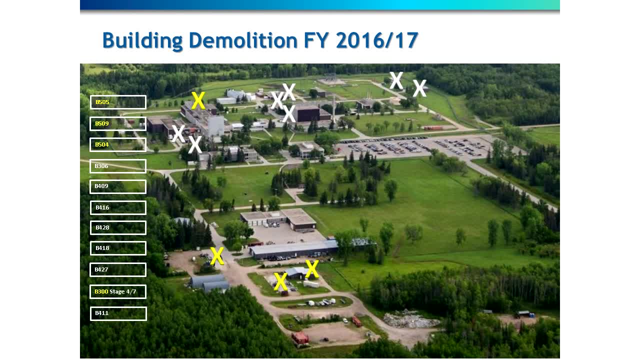 during 2016-2017.. Those indicated in yellow, including building 300, have already been demolished. They include building 300,, as I spoke of earlier, building 505, where soils research was conducted. building 509,, a civil utility test building. 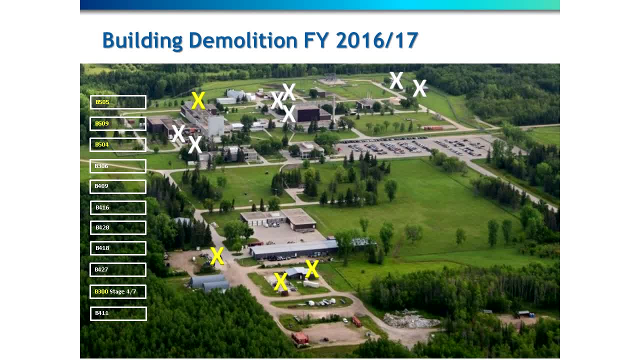 and building 504,, which is used for engineering development and test. The other buildings with the white Xs are planned for this year. They're mostly non-active support facilities, with the exception of building 411, which is in the upper center part. 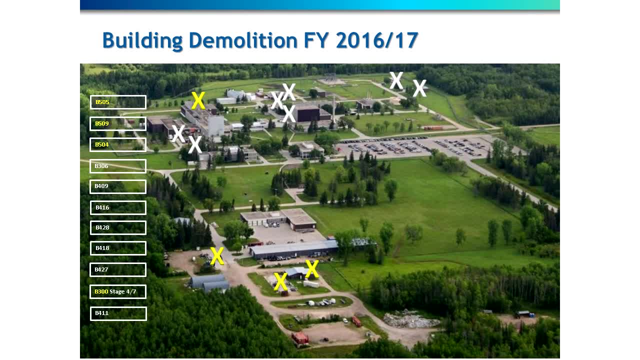 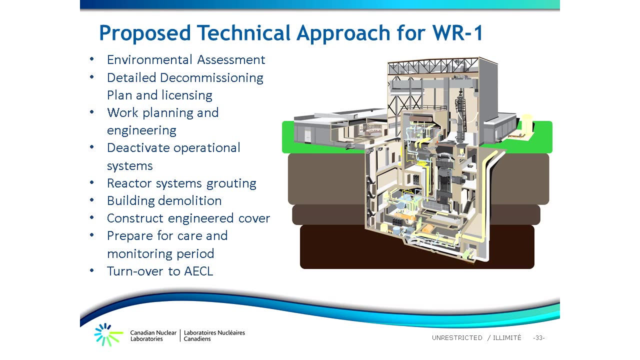 and that is the former decontamination center at white shell And that is currently operationally cleaned and we're continuing with scoping surveys prior to demolition. Turning now to the WR1 reactor, as shown on this slide, The reactor is the void in the center, below grade. 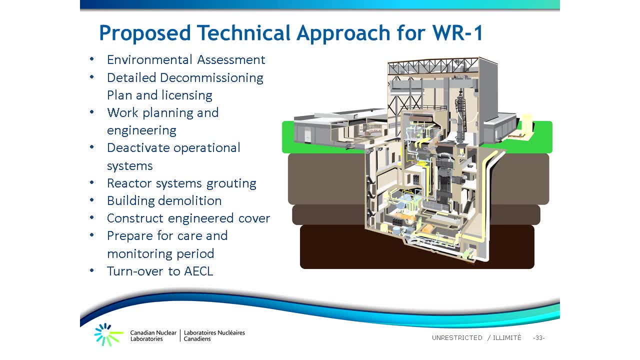 as depicted in the picture, The nuclear systems below grade are in a concrete containment, which make WR1 a good candidate for entombment or in situ decommissioning, which is our proposed approach. The general characteristics of the reactor are the following. 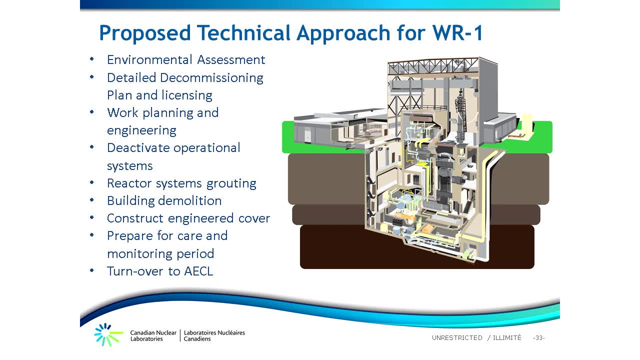 We're going to take a look at some of the components that we're going to take a look at. The components of in situ decommissioning have already been covered by Pat, so I'm not going to repeat them. The section below grade: 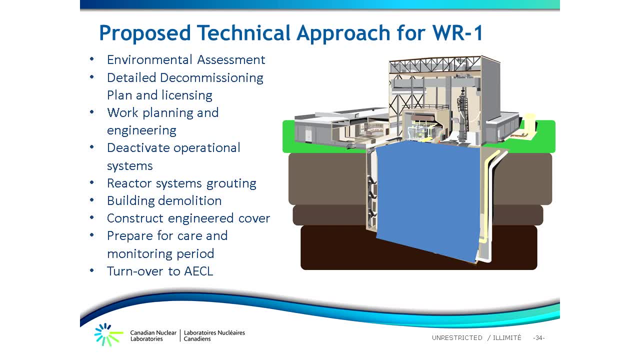 shaded in blue on this slide will remain at the site as is, but encased in grout covered with an engineering cap to contain underground structures. The specific grout will be tailored for the specific characteristics of WR1.. This slide summarizes the methodology. 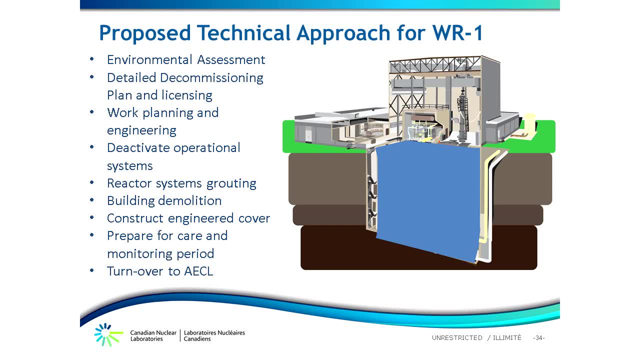 we propose to follow for decommissioning of WR1.. It consists of the following steps. Environmental assessment has been initiated and is currently in progress. We will develop a detailed decommissioning plan detailing our approach. It will be submitted to CNSC staff. 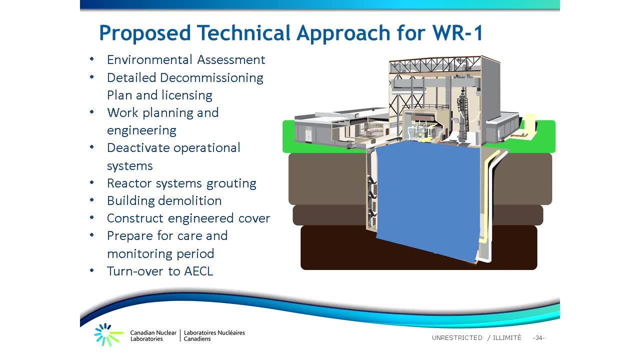 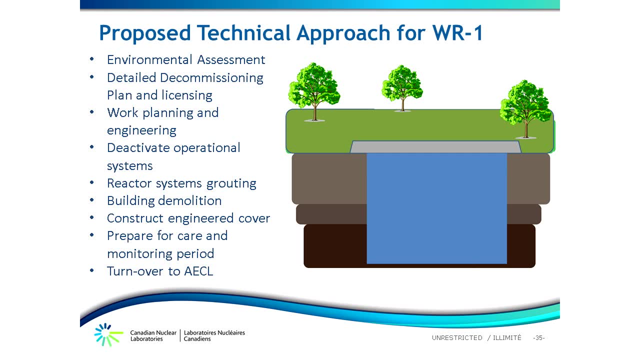 for acceptance through the normal licensing process. The next phases in the process will include work planning and engineering. deactivation of operational systems. grouting reactor systems in below grade areas. demolition of the above grade structure and construction and emplacement of the engineering cover. 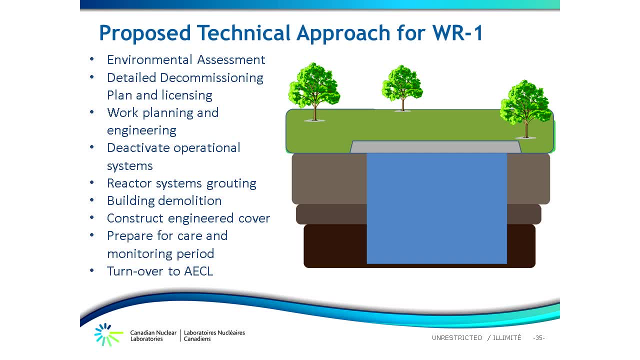 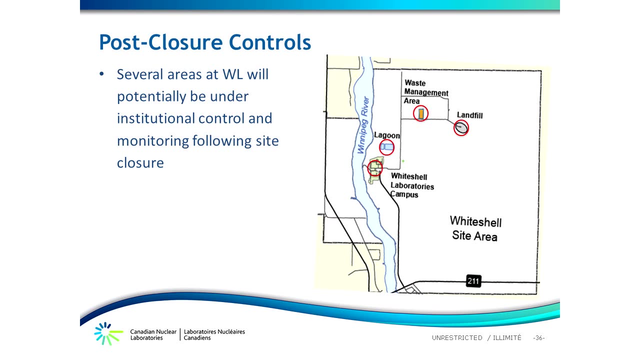 engineered cover. Ultimately, the entombed reactor is planned to be covered in landscape to blend in with the surrounding environment, as depicted on this slide. Once the site has been closed and all decommissioning is complete, there will be several areas at Whiteshell. 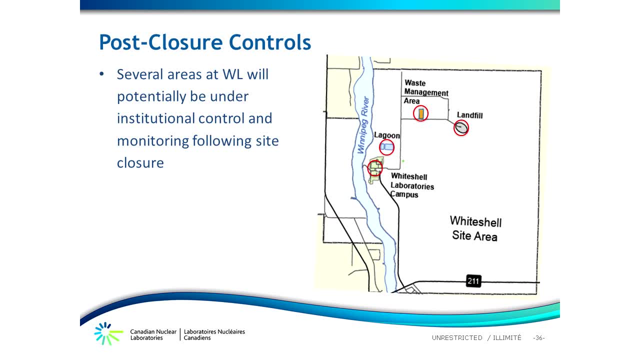 that will be will potentially be under institutional controls and monitoring following site closure. This slide shows potentially impacted areas at the Whiteshell site, including, but not limited to, the landfill, the waste management area, the lagoon and the main campus, which contains WR1.. 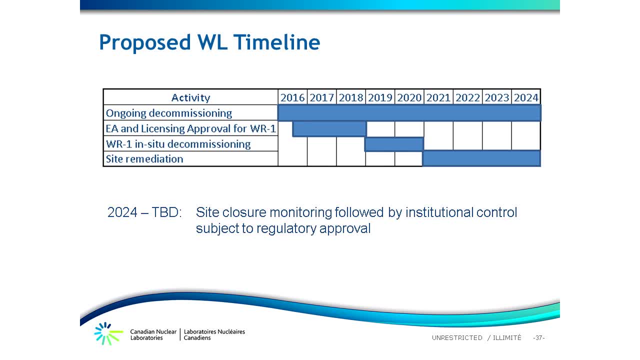 The target timeline shown on this slide indicates our proposed objectives of achieving closure of WR1 by 2020.. Decommissioning of all other buildings and site remediation activities are planned to be completed by 2024.. At that point, the site will be declared closed. 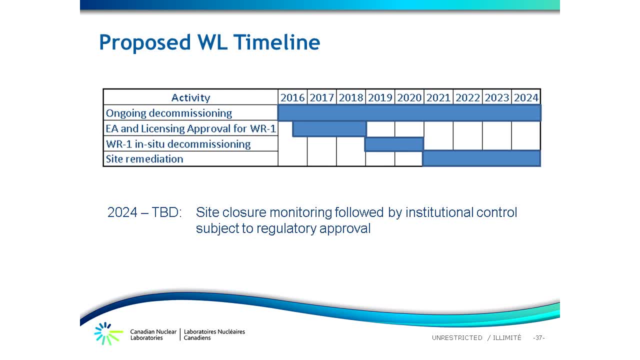 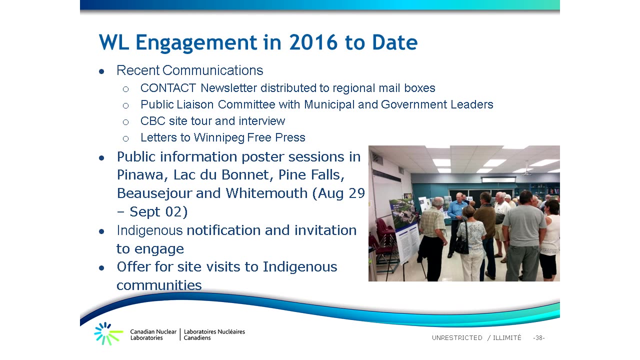 and a period of institutional controls would follow. The end date for institutional controls is to be determined through regulatory action- regulatory process. excuse me, Our CNL team at Whiteshell has been busy throughout 2016 coordinating and conducting local engagement activities. This slide provides a summary of these activities. 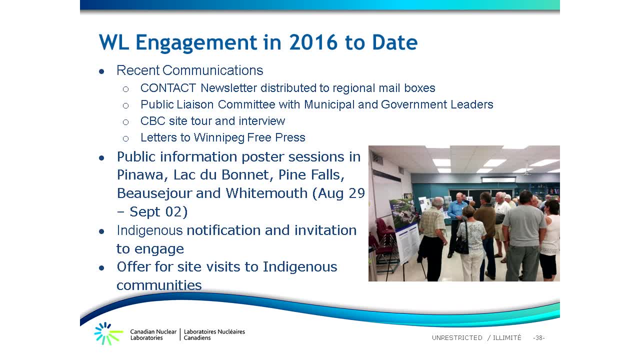 We're proactive in communicating with the public through newsletters and our public liaison committee. We are responsive to requests for information and tours, as demonstrated by the site tour given to CBC Radio Canada and our response to letters to the press. We have held multiple public information sessions. 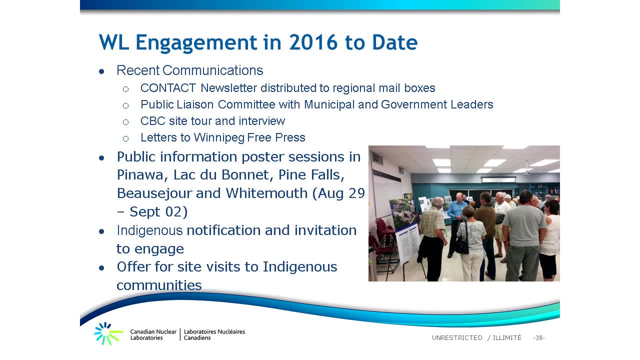 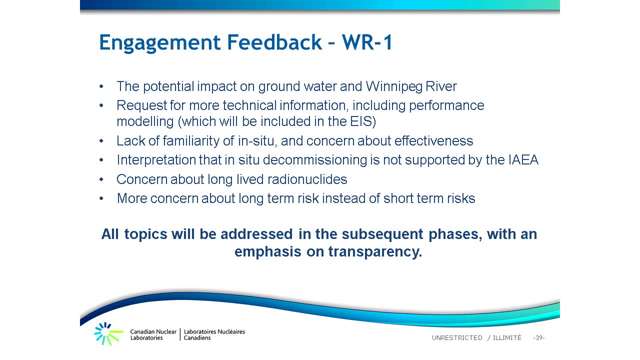 in the local community and are engaging with indigenous communities to ensure they are aware of information that is available and opportunities to visit the site. This slide summarizes what we've heard from our engagement activities to date. The feedback is similar to what was received at MPD and NSDF projects. 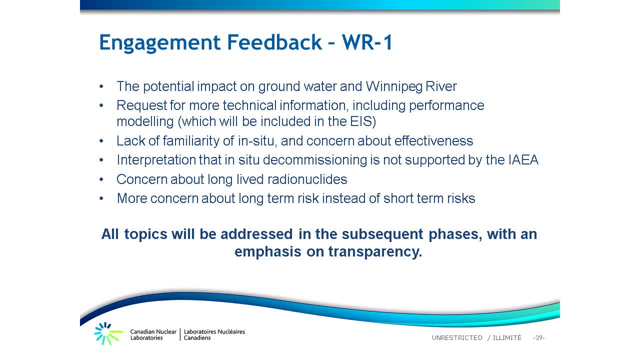 with some additional specific feedback that's unique to WR1 and the Whiteshell site. We are committed to ensuring that our engagement activities are accessible to the public. We will address all of these comments during the environmental assessment process and during further open houses. We will continue our engagement campaigns. 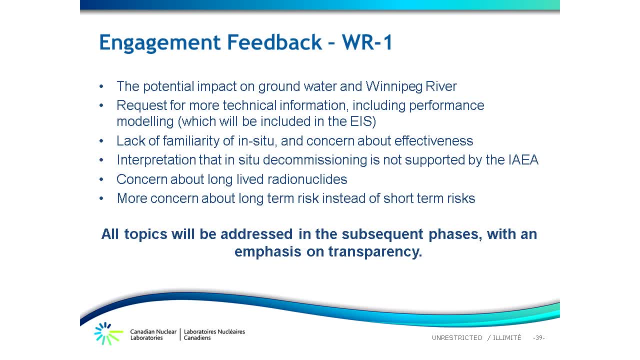 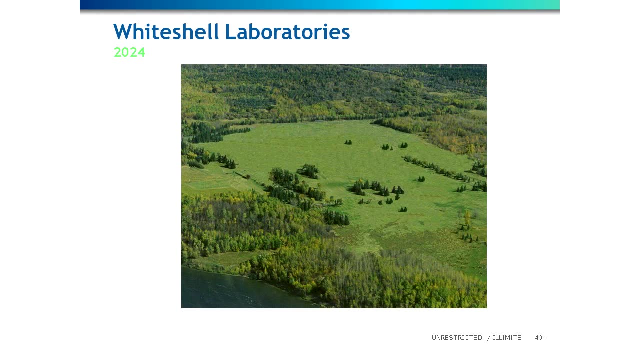 throughout the course of the project. I'm going to end my part of the presentation, but not without showing this slide here. This is our vision of Whiteshell site in 2024.. Note: this does not include institutional controls that could be in place. 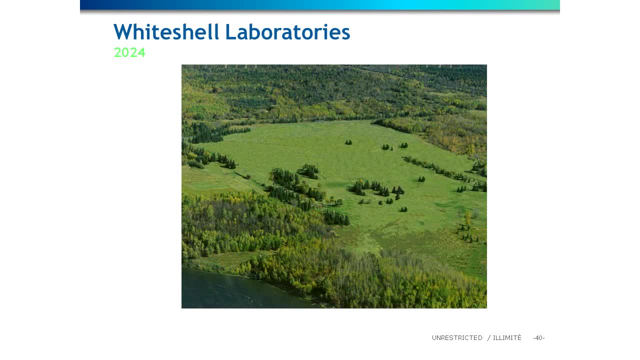 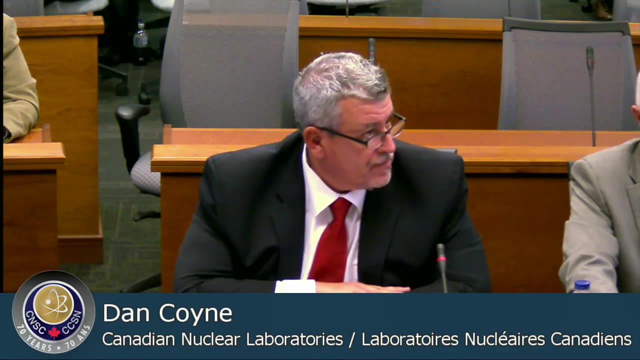 nor any future regrowth opportunities that we are engaging with the community on. Our measure of success will be completing this work safely and leaving a solution that's protective to human health and the environment. With that, I will now turn the presentation over to Mr Keeler. 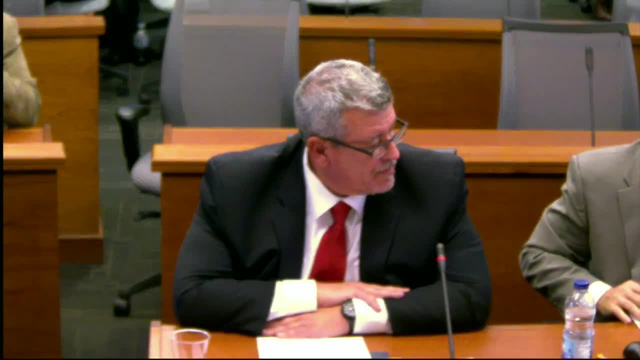 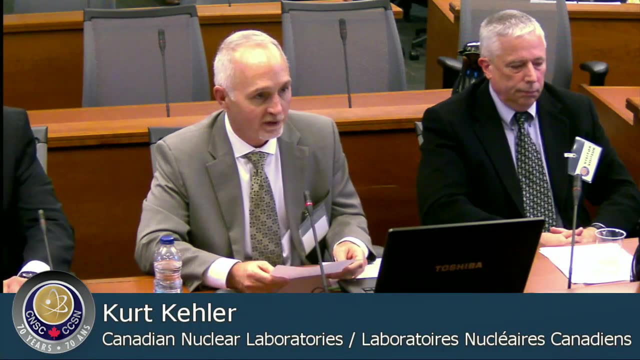 Thanks, Dan Kurt Keeler, for the record. Our goal today was to describe the new mandate for CNL's Decommissioning and Waste Management Organization and how we've responded to it with a new vision and clear strategy for that vision Through all our activities. 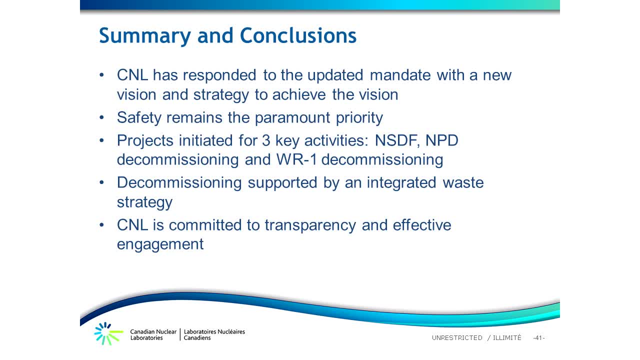 safety remains our highest priority and always will. We have described the three most significant early projects: the Near Surface Disposal Facility, the project to decommission the NPTE reactor at Ralfton and the acceleration closure of the Whiteshell site. 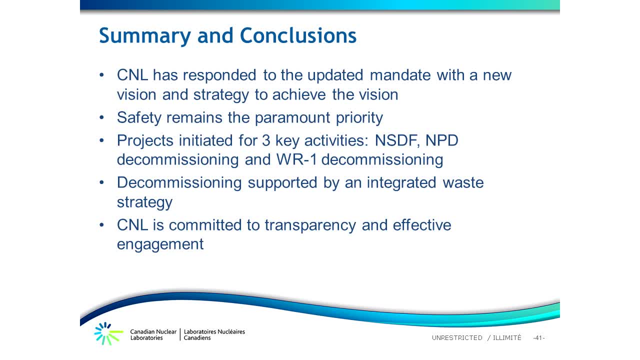 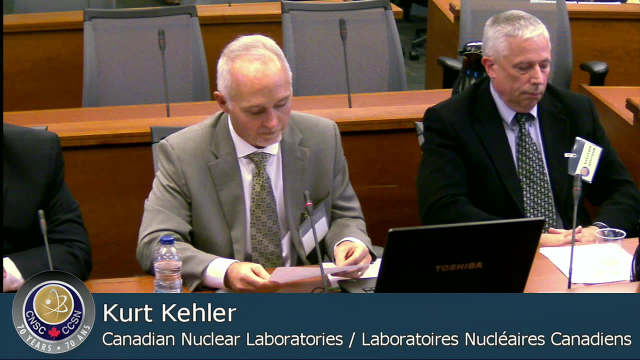 We have also described how our decommissioning activities are supported by an integrated waste strategy. Finally, I want to emphasize that CNL is committed to transparency and truly meaningful engagement throughout all of our activities, including the decommissioning and waste management. Thank you very much for your attention. 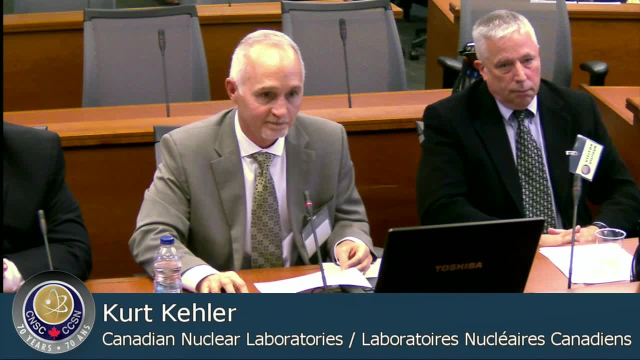 and we'd be happy to address any questions at this time. Thank you, Subtitles by the Amaraorg community.